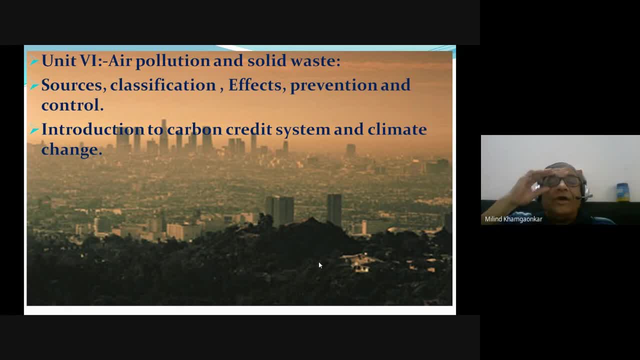 Regarding all these things, we are very much aware only with a type of revision and if some new knowledge is there that is to be gained Again, as I have told you in my first lecture and other lectures to come, that all this environmental engineering too, is again related to your final year elective subjects. 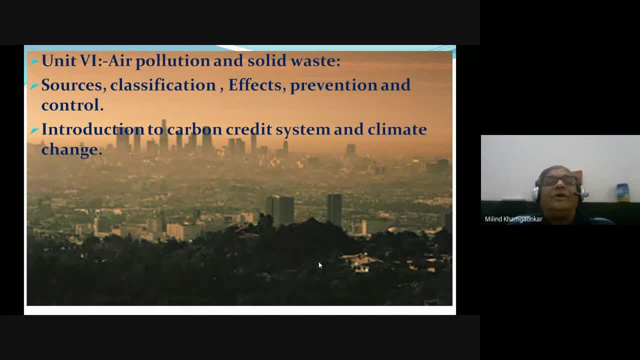 One subject is there which is regarding air pollution. We have only one unit here, Half unit, but one subject is there Also: solid waste management is another subject. you have elective And water and waste water treatment, WWWT In that name. also there is another elective subject. 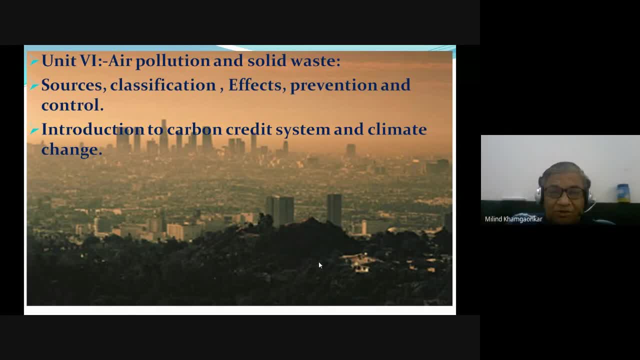 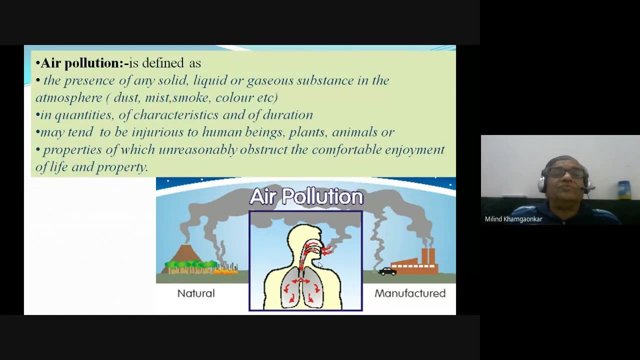 So at this juncture, if we give proper concentration, it will be definitely useful to you in your final year also, And all these notes also. So let us move into the subject without wasting further time. Air pollution: its definition. 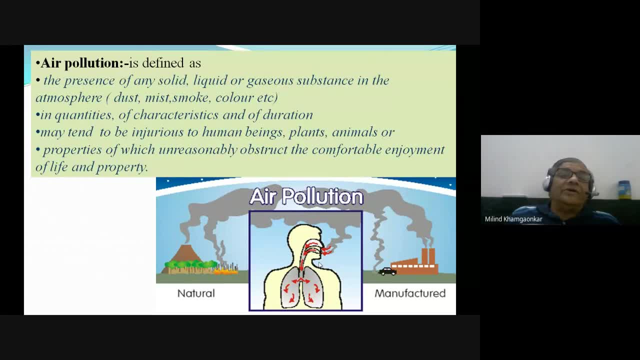 Though we are aware about the air pollution and their effects, etc. Let us see how it is defined: The presence of any solid, liquid or gaseous substance in the atmosphere, That is, dust, mist, smoke, color, etc. I will again repeat: 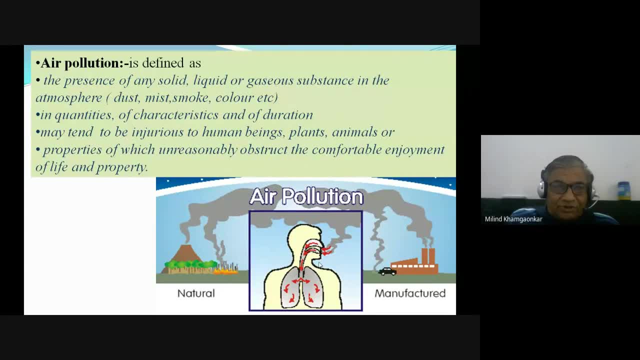 The presence of any solid, liquid or gaseous substance in the atmosphere May be in the form of the dust, mist, smoke, color, various colored smokes, etc. All these are, if present in the atmosphere, In the quantities. Now, in what quantities? 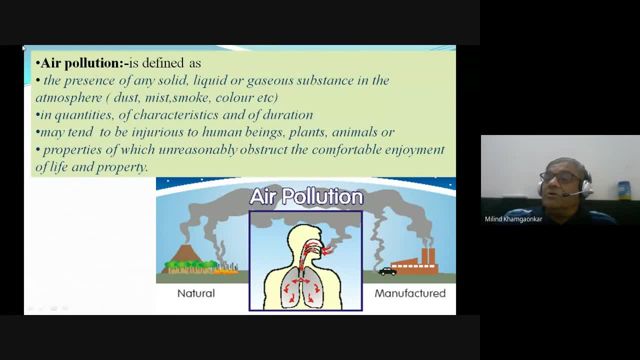 In the quantities, of large quantities, so that its characteristics and duration Means the characteristics and duration of this waste material if it is much more in quantity, and time Means the characteristics and duration of this waste material if it is much more in quantity and time. 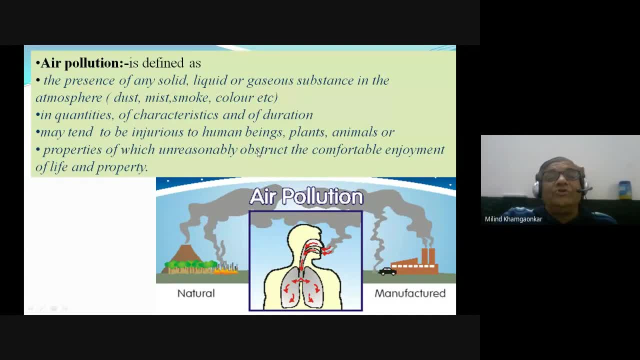 It may be injurious, it may tend to injurious, to human beings, plants, animals or any properties. It may be injurious, it may tend to injurious, to human beings, plants, animals or any properties, Buildings, the agriculture, farms, etc. 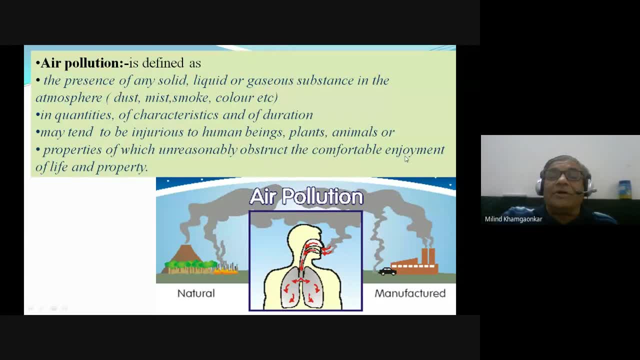 Of which unreasonably obstruct the comfortable enjoyment of life and property. We will again repeat it: Initially, it may feel difficult to understand. Initially, it may feel difficult to understand. Initially, it may feel difficult to understand The meaning of. in short, the meaning of this definition is that 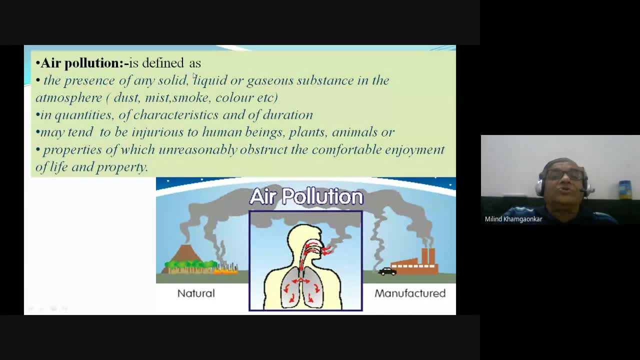 When the particles? solid particles may be in the form of very micro particles, In the suspended form, colloidal form, liquid or the gaseous substance, But much in quantities In the Atmosphere. Their presence in the atmosphere around us. 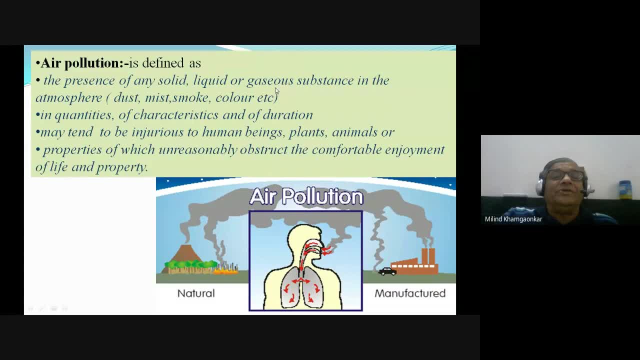 Their presence in the atmosphere around us is much in quantities and their characteristics means, if they are present in the atmosphere and they are showing their properties and characteristics to thus human beings or to the animals or to the plants, and they are for much more duration, then they will be injurious to the human beings. 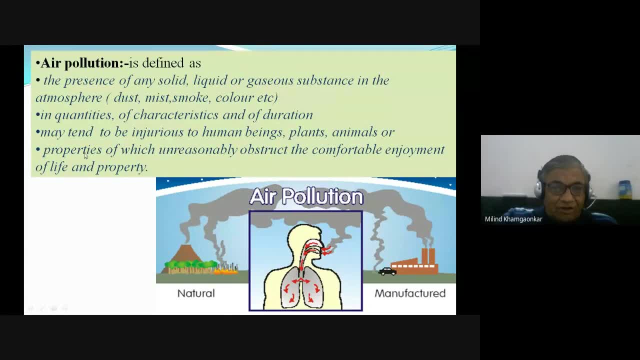 plants, animals, etc. and the properties and which will result in the obstruction of comfortable enjoyment of life and property any in chijo k current hum Joe normal life, jeer a one normal life co kina k to be it is creating obstruction or a danger. all this. then we say that that air is polluted or air pollution is there in. 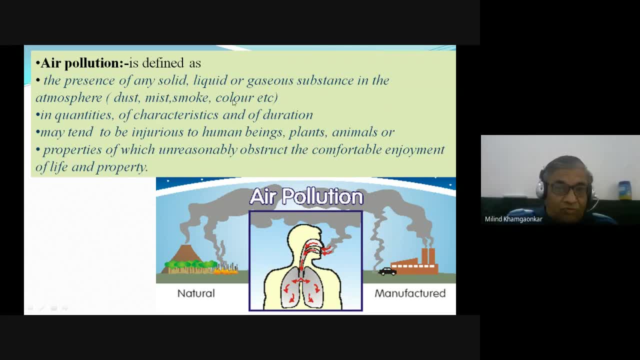 normal surrounding around us. now up sub logo: kaju baju Joe, hey, what he K? ABM sauce, less active plants, a charge. I was up to a problem night. yeah, a building house cook. which name why they kill a car. they were. I saw Jetta, hey. 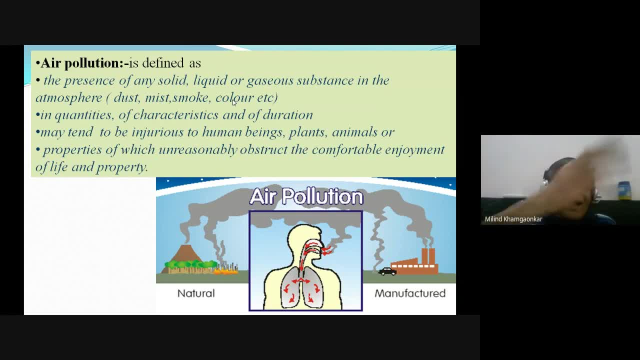 case. sometimes the gas and gas will spread throughout, as the power grid creates a situation where heat can cause the gas to spread and it will cause pollution and that cause the gas to spread all over and the gas will spread. it is something that typically happens in that environment and in our environment. 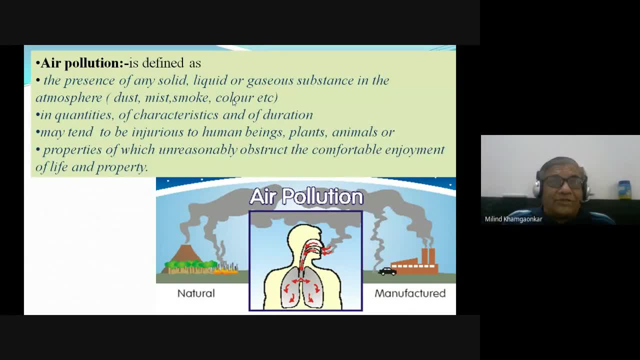 also that on the inside the air can be polluted and that is a gas that has been through, the air passed through and if they do that, all the things they need. you know they might just be slow, but that is a. that is a little bit of a difference, but that is what. this is what we are seeing. people are seeing. 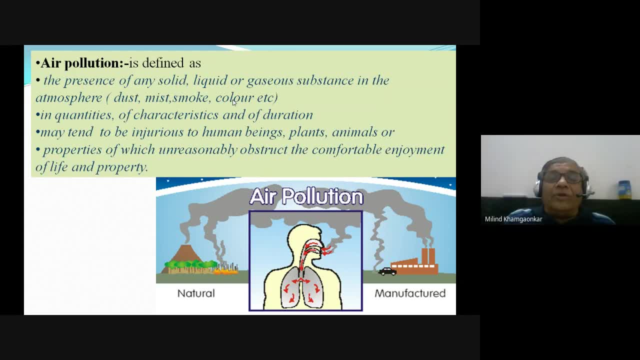 that one side of the earth is really like that the other side of the earth is. And the human beings, animals etc. who are there in that atmosphere, they cannot inhale the oxygen from the atmosphere. They have to inhale that polluted ammonia or chlorine etc. 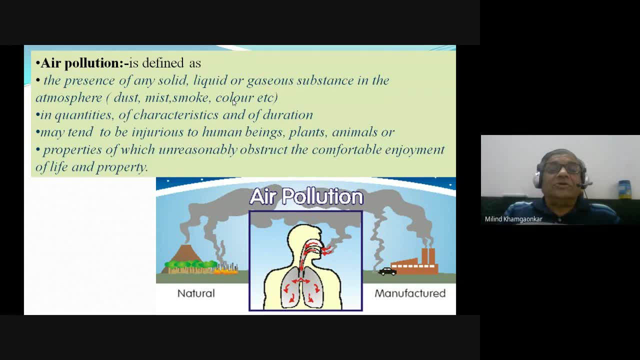 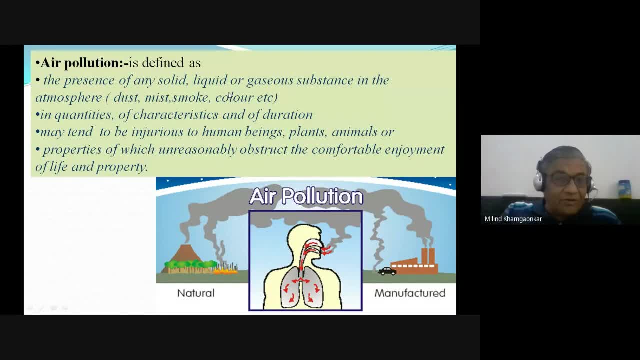 So we all know that all those explosives, they are injurious to the atmosphere. So we all know that all those explosives, they are injurious to the atmosphere. So that is the example, what I mean to say. If we go further, there are plants, plants, etc. 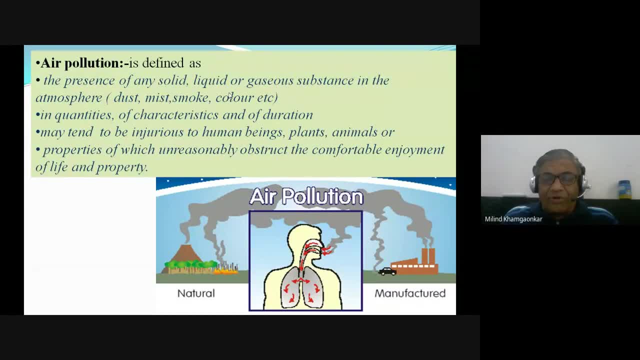 Like I said, Koradi is a thermal power plant. there are many thermal power plants And a lot of the industries are there. What is that? It is a plant that produces fly ash, And the density of that fly ash is so low. 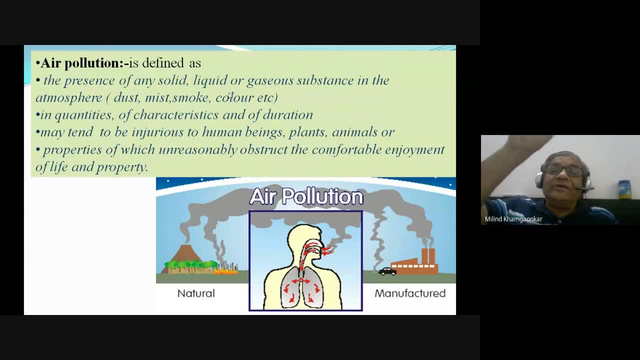 less than the atmosphere, air, etc. It floats and flies into atmosphere and slowly, when the air feels less, it settle around that plant. So it has been observed that around three, four, five, ten, seven, eight, seven, ten years ago. 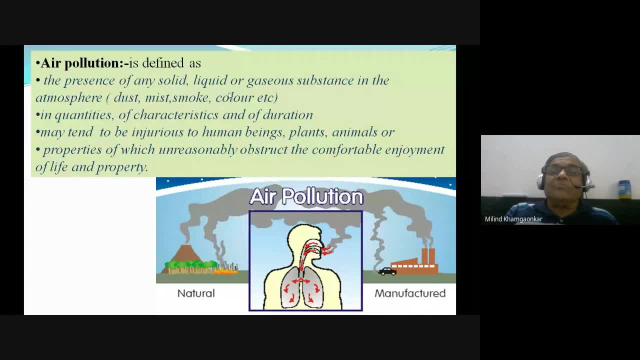 5-10 kilometers around these thermal power plants. The human beings. first is the human beings. they inhale this air containing the fly ash and they have the problem of Asthma that is called as the Dhamma, as well as TB. 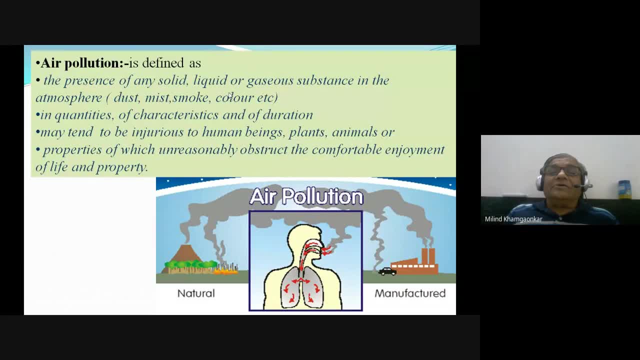 It has been surveyed and found that such plants have this problem, the people around the people, the animal and the human being, as well as agriculture, which is the fields around it. the fly ash accumulates on the fields, on the leaves of the plants, and that also gets affected. 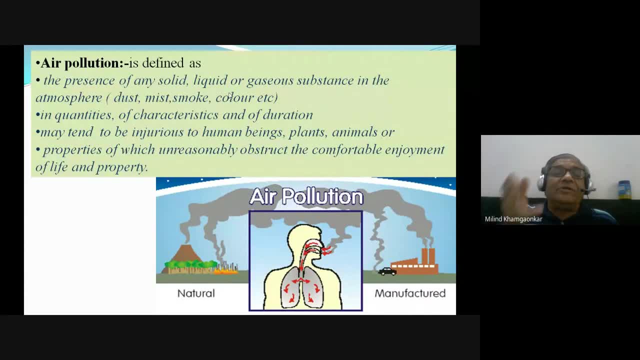 So that you can say the plants, animals, human beings. There is one petrol refinery is there. That refinery emits a lot of the acid gases, the gases containing acids, And the air, the flow of the air, in such a way that the air flows from Mathura to Agra. 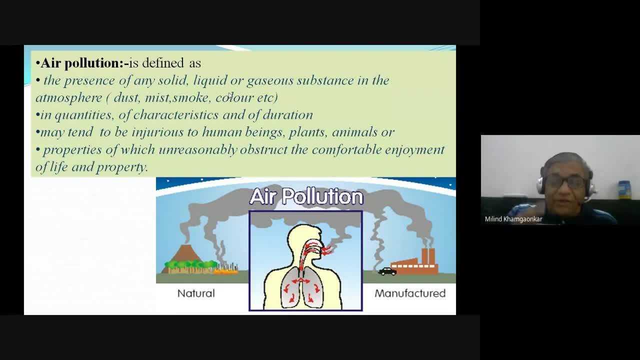 from Mathura towards Agra And it is spoiling the white color of the marble of Taj Mahal. So that is the example of the destruction due to the air pollution to the properties. Okay, So human beings, plants, animals and properties. 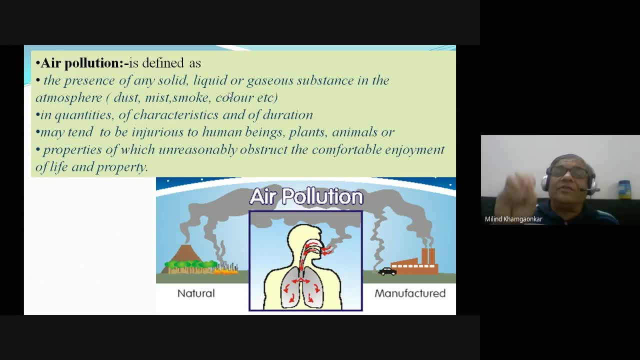 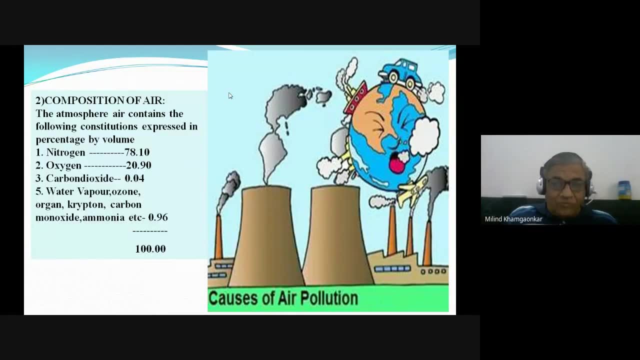 are reasonably get obstructed or they cannot live their comfortable life and enjoyment. Then we say that there is a air pollution. Okay, Now let us move further. What is the composition of air? What is there in the air? The atmospheric air contains nitrogen. 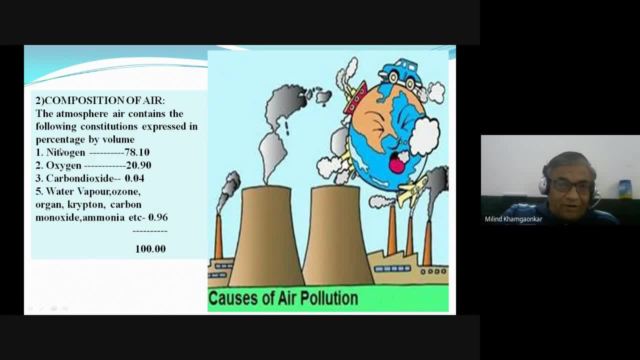 normal air, non-polluted air, contains nitrogen, 78.1% oxygen, almost 21% carbon dioxide, 0.04% and some. the other remaining part, about less than 1% or 0.96, is water vapor, ozone, oregon, krypton, carbon monoxide. 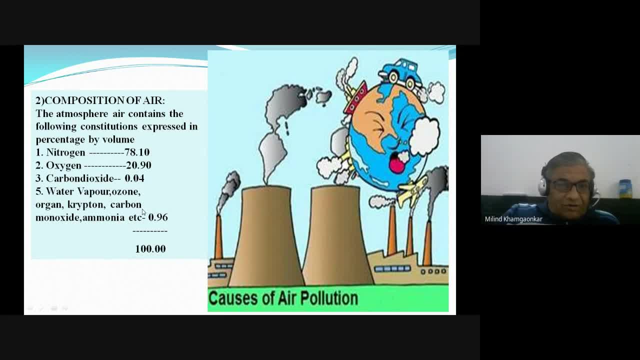 Ammonia, et cetera. Okay, So these are the things which are present in the normal air, But when this balance loses or imbalance occurs due to the extra presence of the carbon dioxide or carbon monoxide, or some ammonium or any chloride vapor, pollution contents. 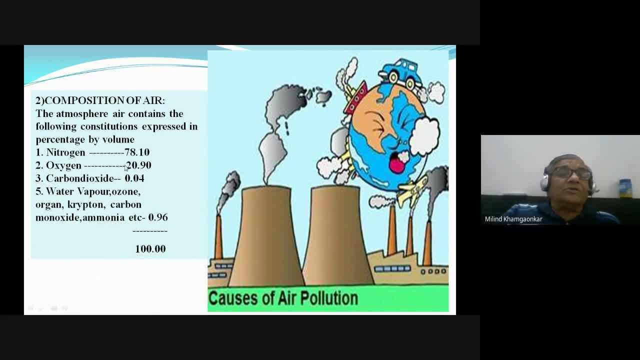 then this imbalance occurs, the oxygen level reduces, and then the human being, the plants, et cetera, all those gets affected due to this imbalance, For which, again, the main cause, as you can see on the right side, is the human being. 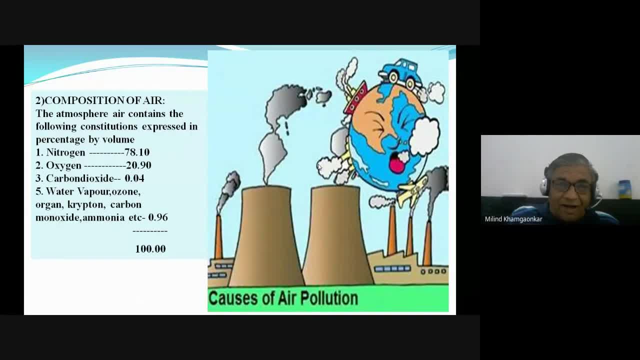 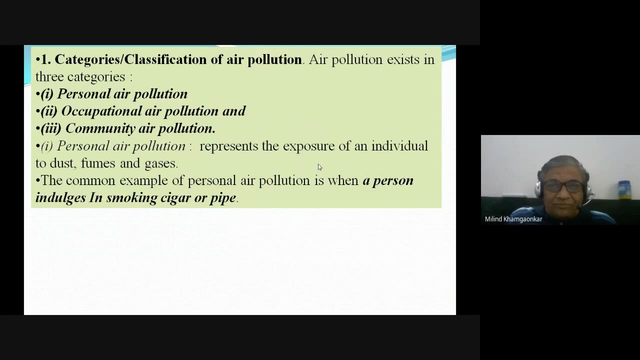 Natural, we will see in the later slides to come what are the various causes. So we can see there. Okay, So let us move further Now. various categories or classification of the air pollution. Air pollution exists in three categories, or air pollution is classified in three parts. 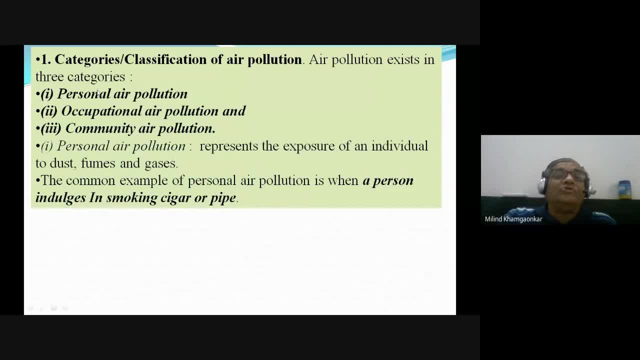 three categories. The one is the personal air pollution, Second is the occupational air pollution And the third is the community air pollution. We are not learning any new thing, Only the knowledge which we have, or the general knowledge which we have. we will be just categorizing it. 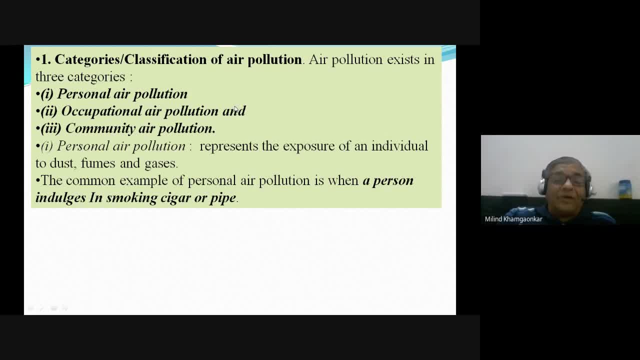 or arranging it in systematic manner, which is also there in your syllabus. The questions are asked on this. So, therefore, the categories or classification of the air pollution- personal air pollution, occupational air pollution and third is the community air pollution. Okay, 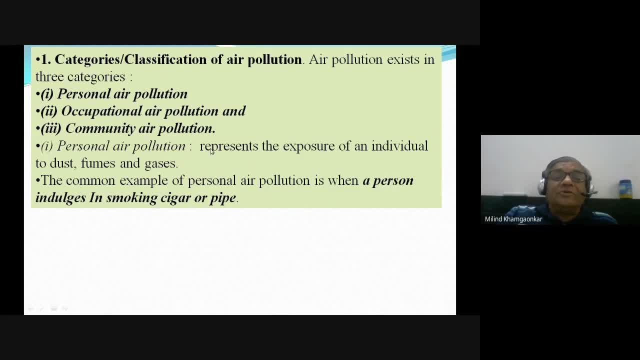 So let us see one by one. Personal air pollution represents the exposure of an individual to dust, fumes and gases. Personal means when a person gets affected due to the pollution of air. then we can call it as the personal air pollution. 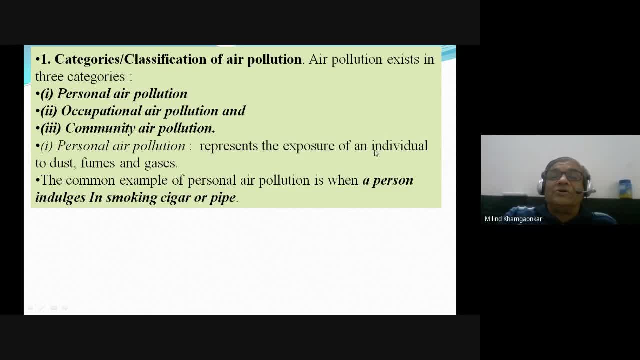 wherein the person is exposed to the dust fumes- again a sort of the dust and water mix, or some hot gases and the gases, That is, the various carbon dioxide, carbon monoxide, ammonium, etc. Now, the common example of this personal air pollution. 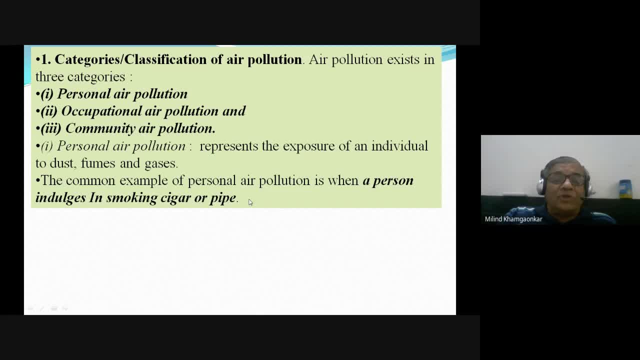 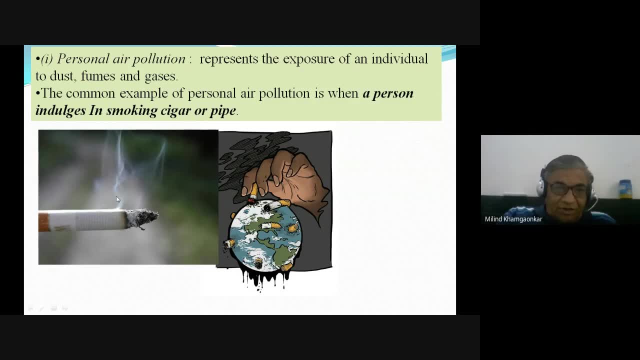 is when a person indulges in smoking cigarette or the pipe, When we inhale, when we take cigarette, in personal air pollution, so that cigarette not only transfers the carbon dioxide gas to the person who is enjoying the cigarette or who is smoking, that smoker gets as affected. 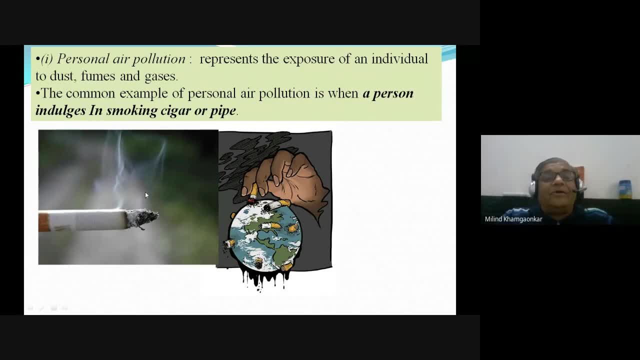 as well as the person who is standing nearby to that smoker. He also gets affected due to the smoke exhaled by the cigarette, And that is more dangerous than the person who is smoking. It is called active or passive smoker. Active smoker means the one who smokes. 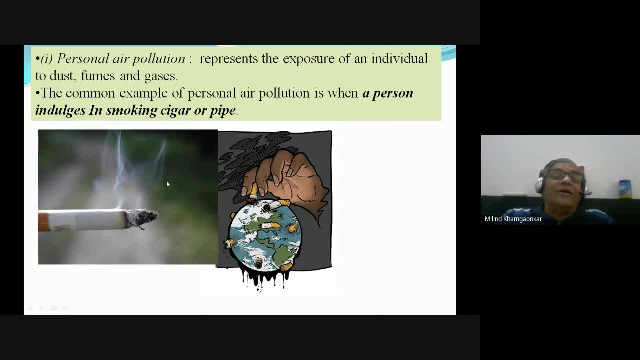 and passive smoker means the one who does not smoke but stands near the smoker, So he is more affected than the cigarette smoking or the personal. So that is the example of the personal air pollution. Our whole earth is getting affected due to this. one of the examples. 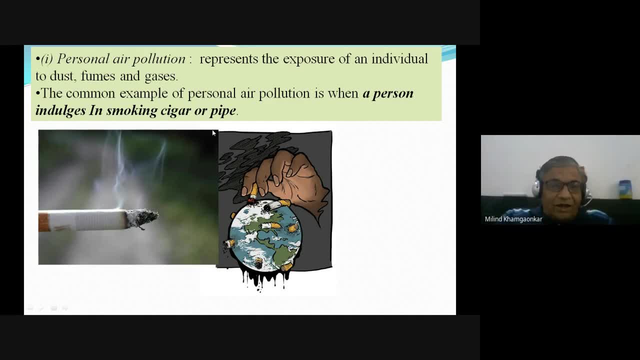 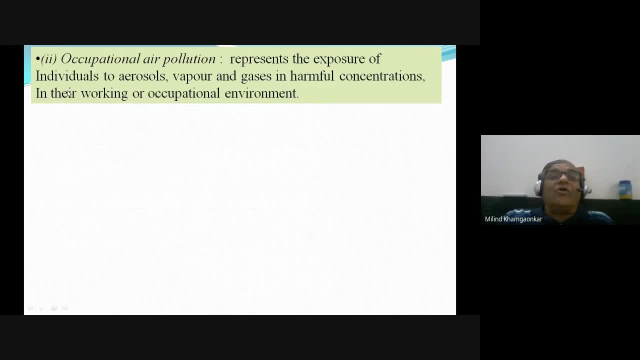 There are numerous other than this cigarette. There are, again, numerous examples of the personal air pollution, But this is one of the examples. Second is the occupational air pollution. Represents the exposure of the individual to aerosols, vapour and gases in harmful concentrations. 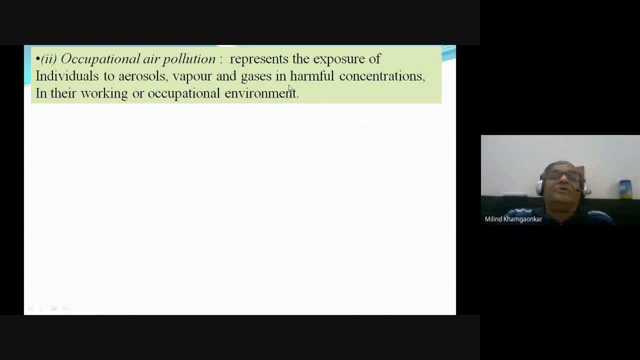 in their working or occupational environment. These aerosols, vapours and gases are again the pollutants. We will be learning all those pollutants, or the things which are which pollute the atmosphere. They are called as the pollutants Aerosols, Very, very fine. 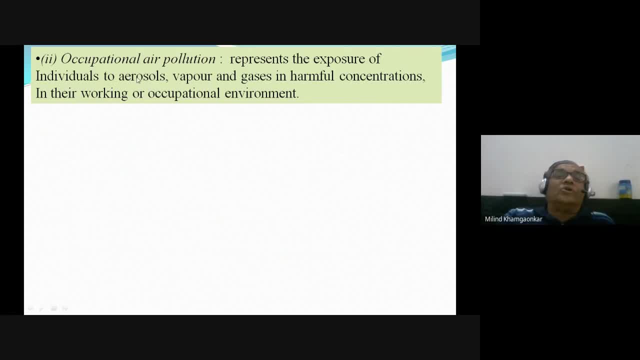 which remain as tantu or threads. They are called aerosols. They are dust particles. These we may not see by our naked eyes. They are not seen by our eyes, But they remain in the atmosphere And if they are, much in quantities, 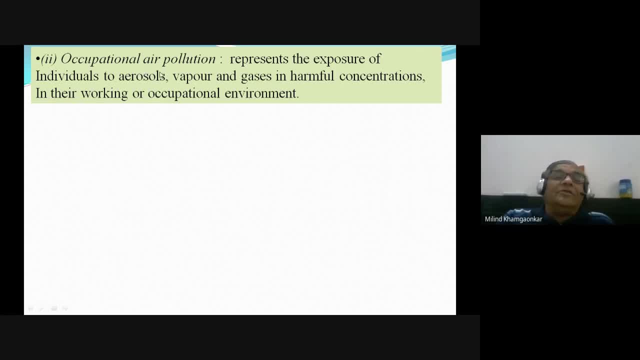 then if they are inhaled, then there is a chances of hazard to our lungs And ultimately spoils our health, As well as vapour And the gases Now where the human is exposed to these things During his occupation. Occupation means where he works. 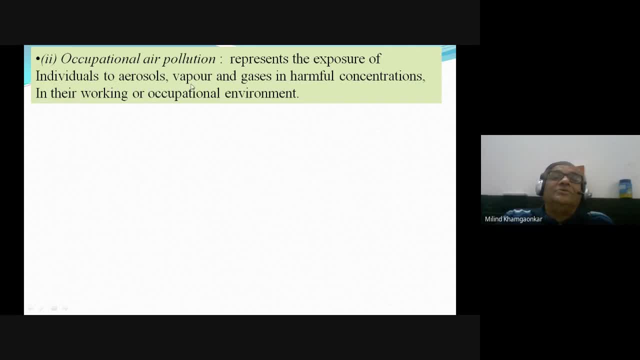 Where he performs his services, Where he does his work. That occupation It is called as occupation. So the pollution in that occupation There is a lot of pollution. There are many such things That a particular fiberglass industry or a particular where fibers are used to make sheets, etc. 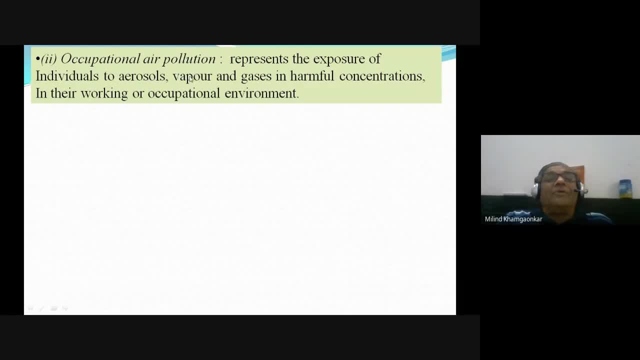 Like asbestos sheets etc. Someone works there, Or a particular works in a particular mine, A particular works in a particular factory, In a chemical factory where vapours and gases are produced, A particular works in a thermal power plant. There fly ash and the water vapour and the steam is there. 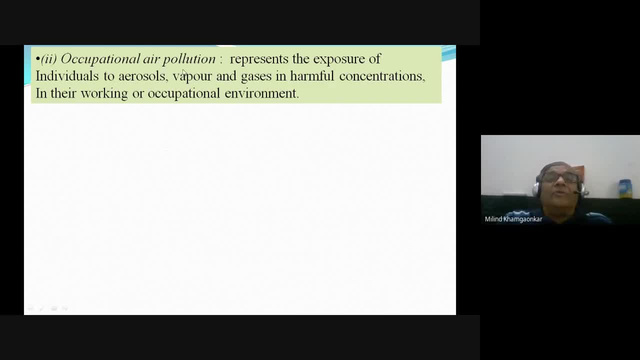 He is exposed to the fly ash, water vapour and the steam. So in that case that person is definitely get affected And his health gets deteriorated. He definitely gets. It has been observed, The survey has been made, That how the occupation affects the person, 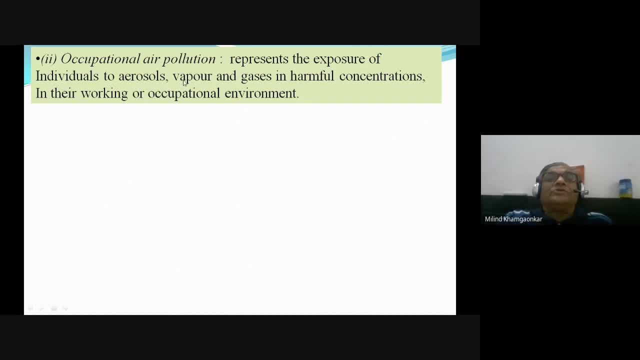 The person's health, All the persons who are working in the different occupations- Some are working in certain pharmacies, Pharmaceuticals, Those pharmacies also gets affected. We get the result. We get the result That the vaccines are coming in the readymade market. 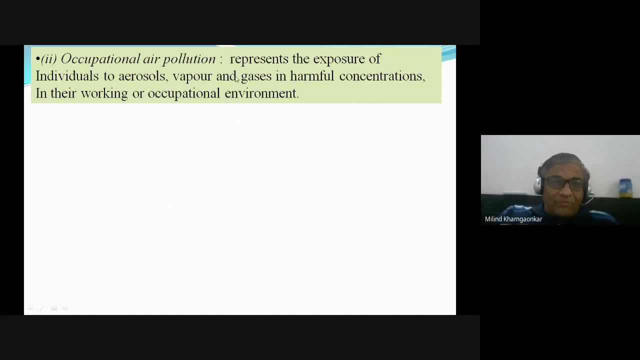 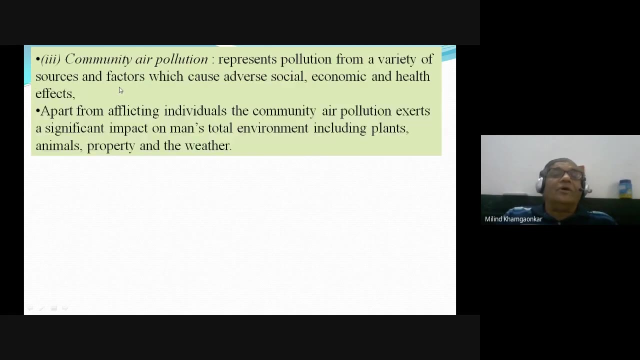 But where this vaccine is produced, Like in Pune, there is Serum Institute Or Bharat biotech in Hyderabad. There the persons definitely get affected. So those are all called as the occupational air pollution. Okay, So this is the example of the occupational air pollution. 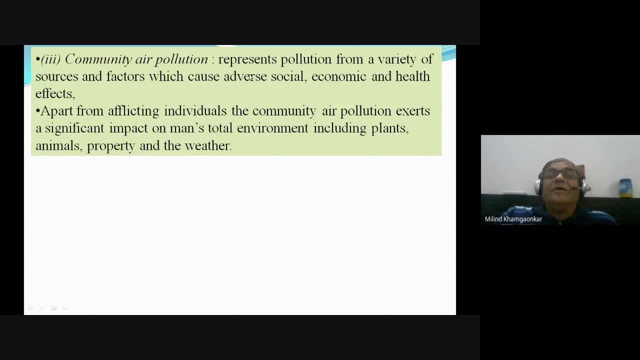 Then the community air pollution. It represents pollution from the variety of sources and factors Which cause adverse social, economic and health. effect Means the pollution that has been created in the society Or in the community. Many a times it happens to us that in the houses we light the stove. 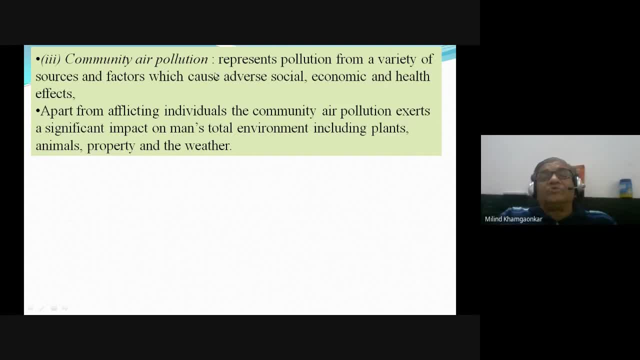 In the villages Or in the city, also In certain slum areas, etc. Unfortunately they could not afford the liquid, That LNG Natural gas, Liquid natural gas, Or that cylinder gas Cylinders. Then the person use the woods. 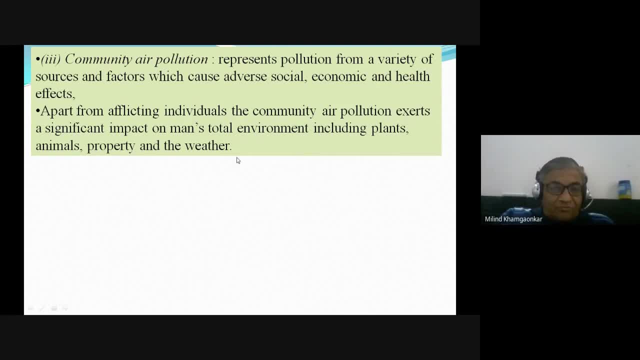 Logs For their combustion purpose, For their daily livelihood. Then also the lot of the pollution has been created Due to the formation of the carbon dioxide, etc. So these are the. This is one of the example of the community air pollution. Another various examples. 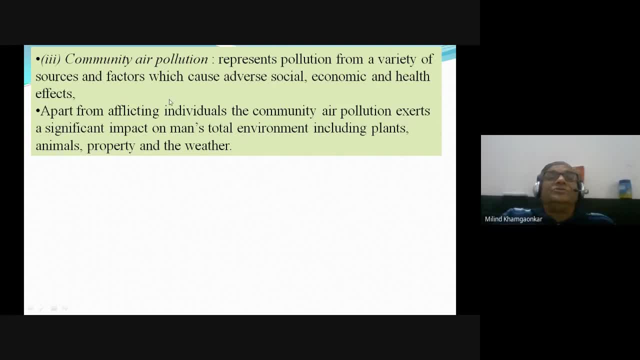 Are there Other than this? If sometimes the community Or the society does not follow the proper Hygiene procedures, The waste material is thrown on the debris In the form of the houses Or in lump at the corner of the roads, etc. 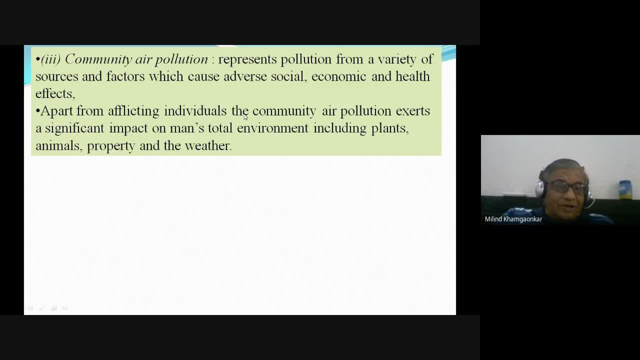 And if it is not disposed properly, Then the decomposition starts And the hazardous gases, Etc. They are evolved from that Combusted Material Or the decomposed material. So that is called as the community air pollution. Now the classification of the pollutants. 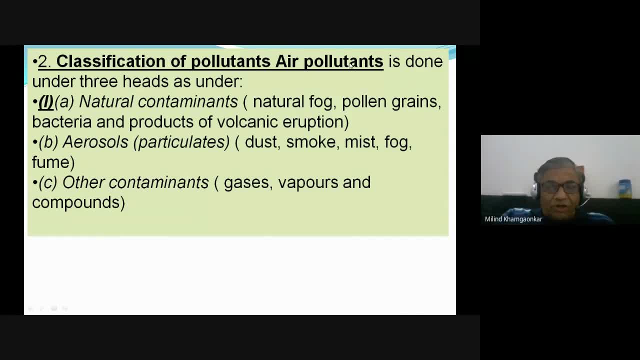 Air pollutants. Okay, How the air pollutants are classified. They are done under three heads. The first is the natural contaminants, natural pollutants that pollute the air, That is the natural today. Those polluted in our control, In the human control. 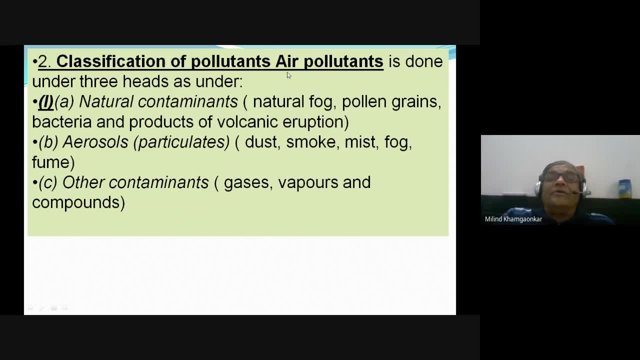 They are the natural fog. ____ غ على. That is the natural tlthi elle The cream. All the time most agua ta season change on Earth. We need the facility from winter to summer Or summer to rainy Season. 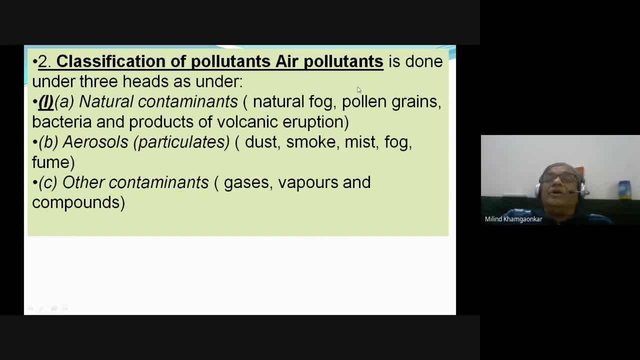 rainy season to winter again. then, due to the change in the season and the temperature and the growth of certain flowers of the plants, the pollen grains start floating into the atmosphere and a certain pollens of the flowers of the plants etc. and those pollens if they are inhaled by the person who is allergic to. 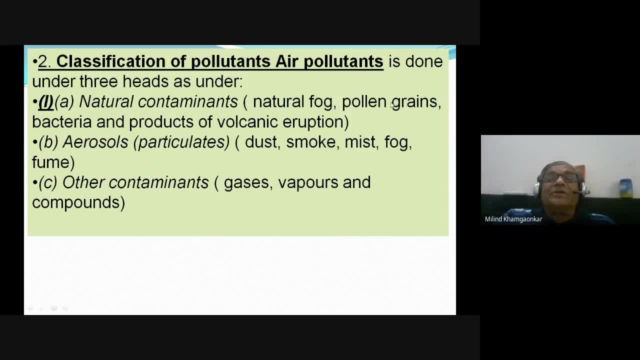 that pollen grains, then that person may suffer by the asthma, or we say that asthmatic attack is there, so that attack is due to the pollution and maybe sometimes in the form of the pollen grains which are available into the atmosphere. then the bacteria there. there are certain bacterias which naturally 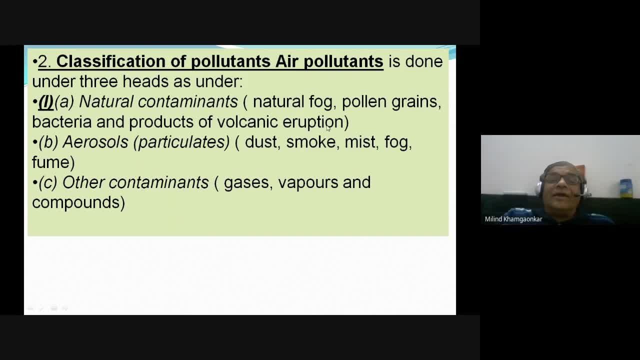 occur into the atmosphere, products of volcanic eruption, volcano you and the volcanic eruptions. these are all the natural contaminants. and the volcanic eruptions, these are all the natural contaminants. then there are certain aerosols. aerosols is called particulate, we both a particulate. this word has come from the word particles, very fine particles which 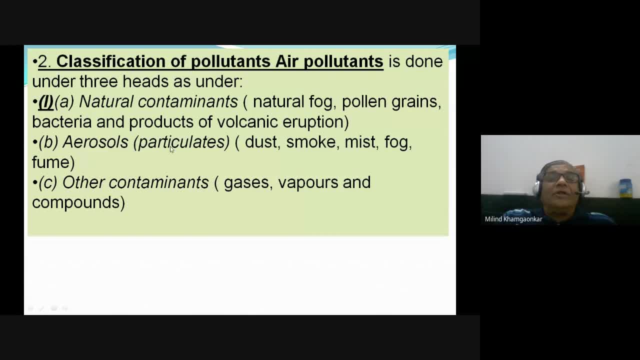 may be seen below the microscope by the, but our naked eye cannot see it. they are called as the aerosols. so these aerosols which present in the atmosphere are Cesur in the form of the dust, dust, dust. actually, due to this dust only we can see our skies blue. you can search on the. 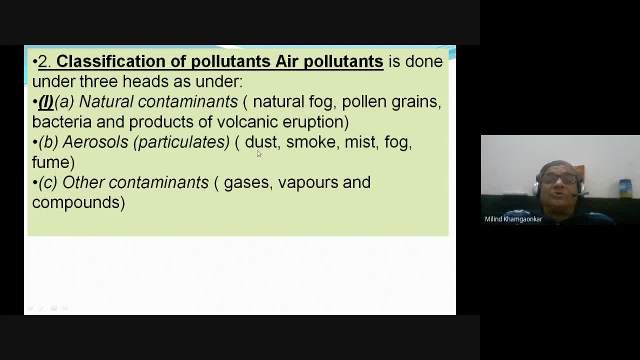 dust. actually, due to this dust only we can see our skies blue. you can search on why the atmospheric skies- I am using the word atmospheric cries- skies around the earth looks blue and a oraz que atmosphere can bar headium jetty black light lights lightingará Wort. 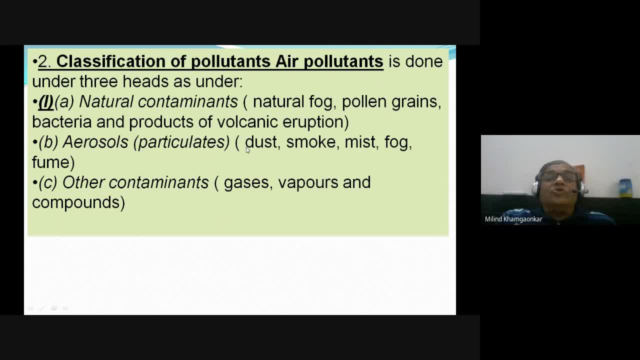 atmospheric offerings- guys- I am using the word atmospheric- imitate Phil Fantine's ajakerate: everywhere is black, no blue or no other color. again we come into the atmosphere of other planet. we will get the colored atmosphere or the skies only due to their dust, because the refraction takes place. refraction of the rays takes place over this dust and due 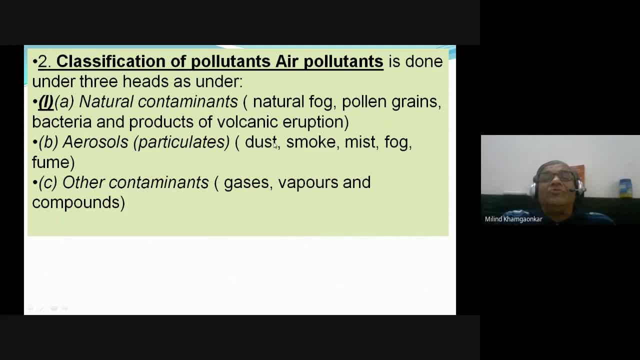 to the refraction, they are converted into the various colors- seven colors you all know- and one of, the blue color, is being seen as the sky for us. so dust is there, but if it is more in quantity then that is dangerous, injurious or dangerous for the human being. 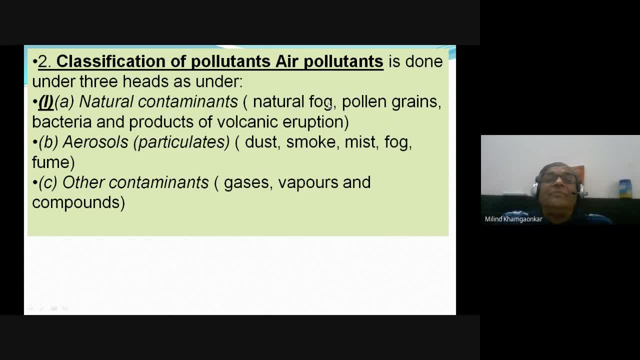 second is the smoke. smoke is there. it may be due to the natural volcanic eruption, but we, the human being, are more responsible for creating the smoke, maybe in the form of the industry, maybe in the form of the four wheelers, two wheelers, three wheelers that we use, okay, and the other automobile. 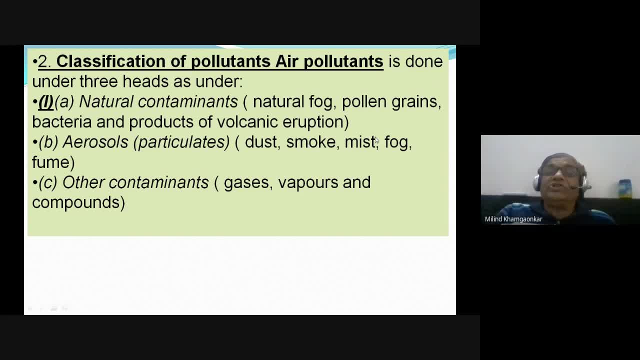 machineries, equipments. mist again, a sort of the fog mist is there. fog is there and the fume may fume again. they are produced in the air from the industries or maybe due to the burning of certain materials. so those are all. those are all responsible for creation of the aerosols. third is the other count: contaminants. 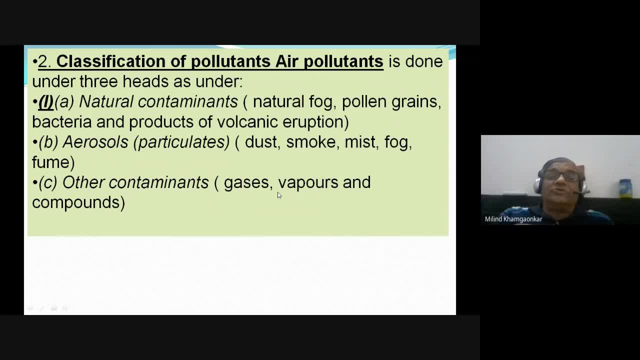 that is, the gases, vapors and the other compounds. okay, so these are all the air pollutants which are present in the atmosphere, or the yellow air pollutants are classified according to their availability into the atmosphere as the natural air contaminants. second is the aerosols and the third is other contaminant. now the other classification. 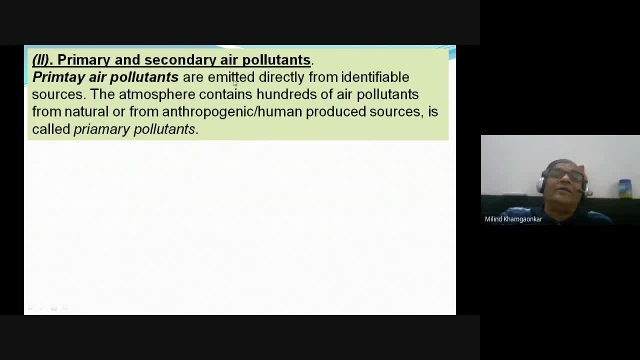 of these pollutants are the primary pollutant and the secondary. other way of classification: primary air pollutants are nothing but they are emitted directly from identified sources. contains hundreds of the air pollutants from natural or from anthropogenic or the human produce sources. is called as the primary pollutants. take a primary in a. 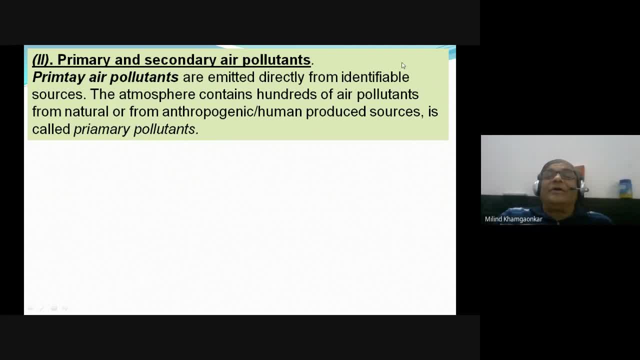 joke directly produce with a high equity sources came at them say, yes, a cool jungle gel raja ya koi khade industry make a explosion over a and up or we volcanic eruption. hey, these are all the primary air pollutants, but with the help of the primary, with the combination of the 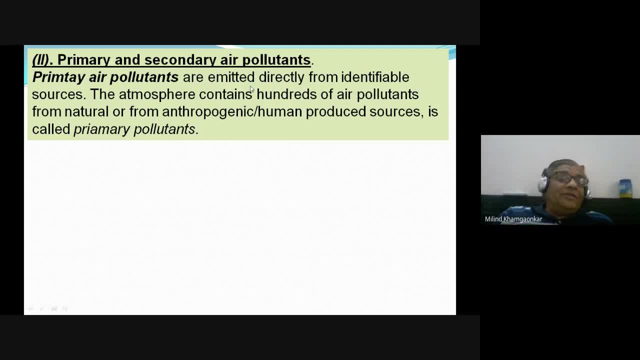 primary air pollutants like the acid fumes or the acid gases into atmosphere and if unfortunately at that time certain precipitation occurs, then this acid fumes or acid gases gets dissolved into that precipitation and we say that acid rain is occurring. so that is secondary air polluted. we will move into that part. so primary air pollutants are: 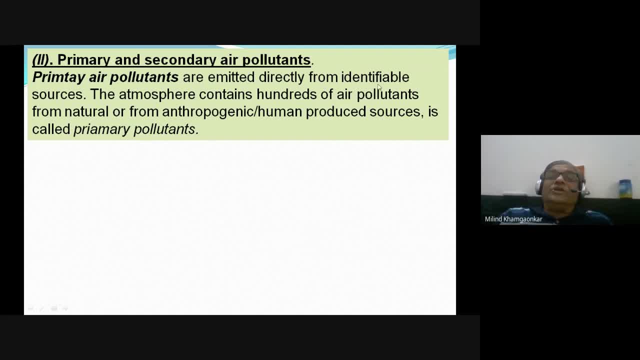 nothing but the original pollution that has occurred from the sources. they may be natural, like the volcanic eruption, or maybe due to the cloud burst. are the thunderstorm cloud burst or the thunderstorm G, samveeg, karadna, kirk, able? and certain human produce sources, like the various industries, the chemical industries, the. 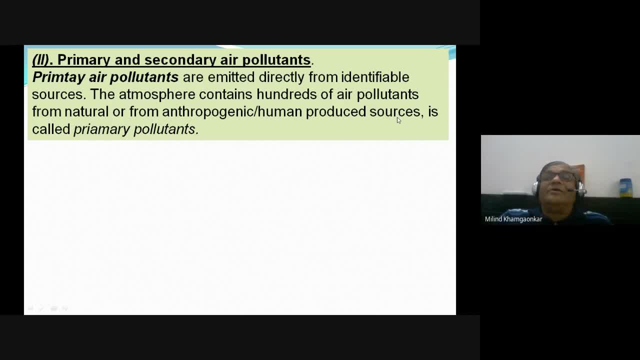 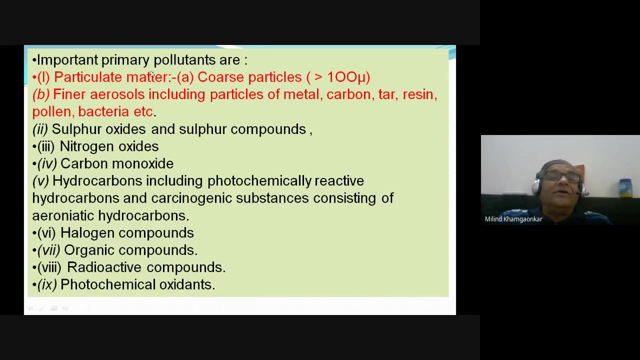 thermal power plants, the steel power plant. they are the main source of the thousands and thousands and crores in quantity of the pollution. they are the primary pollutants. now the secondary poll you. important primary pollutants are: particulate matter, coarse particle which are greater than 100 micron size. finer aerosols, including particles of the. 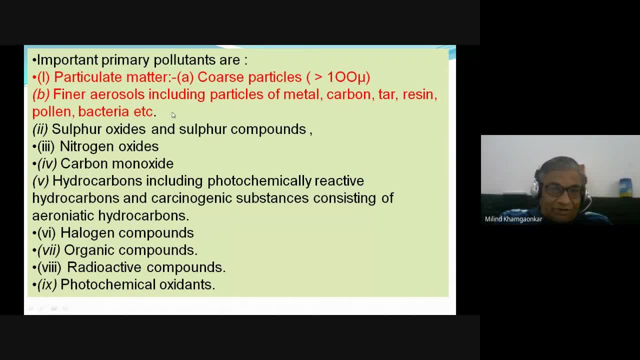 metal, carbon, tar, resin, pollen, bacteria, etc. sulfur oxide and sulfur compounds, nitrogen oxides, carbon monoxide, hydrocarbons, including photochemically reactive hydrocarbon. carcinogenic substances consist of the aeronautic hydrocarbons halogen compound in a chlorine, fluorine, iodine, etc. organic. 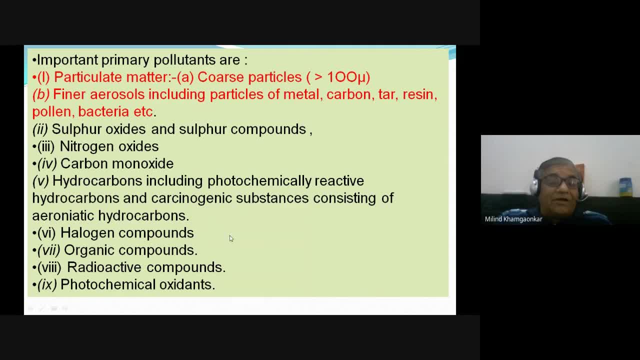 compounds: methane, ethane, acetylene, etc. radioactive compounds: you all know the, all the radioactive materials. photochemical compounds, compounds which are responsible for the photochemicals. okay, so these are all called as the primary air pollutants, which are mainly subdivided into the coarse particles and the finer aerosols, and then further the in the form of the. 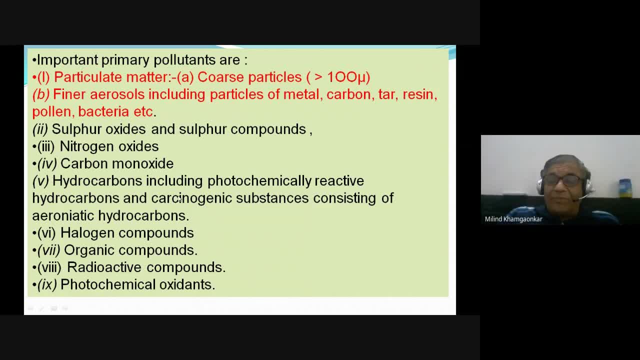 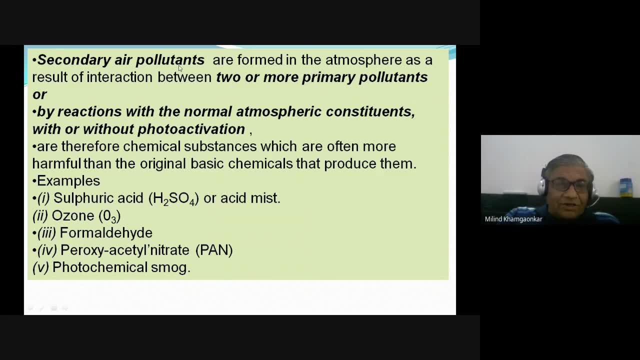 various gases examine. so these are the important primary pollutants. now the secondary air pollutants are formed in the atmosphere as a result of the air of interaction between two or more primary pollutants. when that, yes, your primary pollutant head, yeah, job X, a jada, do job X at mix with the other. now, and 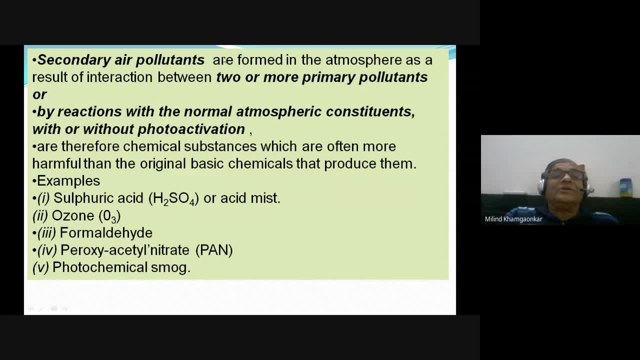 I have a pollution there was at that then that is called as the secondary air pollutant. okay, how this occurs? by the reactions with normal atmospheric constituents, with or without photoactivation, and either two or more pollutants react together, form a third pollutant or, as I have told that the 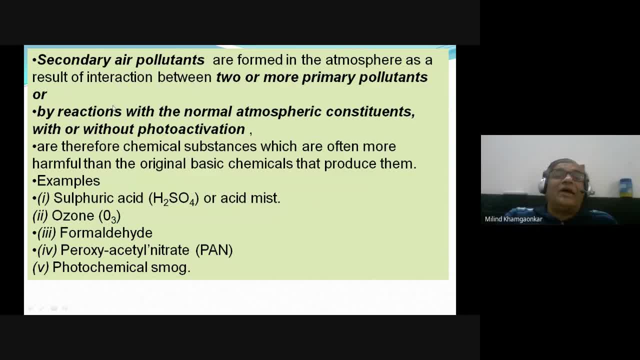 acid present, acidic fumes or gases present in the atmosphere may be from certain industry etc. when it gets mixed with the rain or the precipitation, then that ray, acid rain, occurs. so this is the second example: by reaction with normal atmosphere constituents with or without any photoactivation, therefore they are the 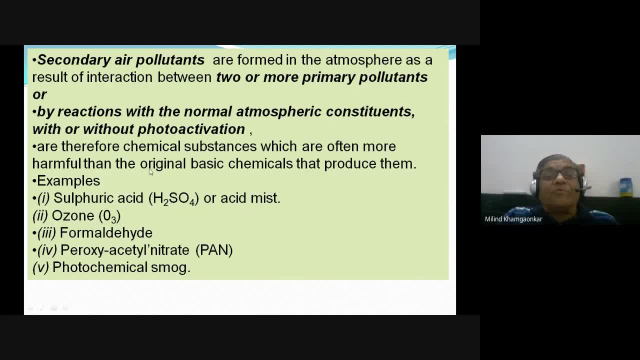 chemical substances which are often more harmful than the organic basic chemicals that produce them in a age, oh hey, don't know. secondary air pollutants- combination of the two or more primary pollutants- are more dangerous than their original pollutants. primary pollutant- joy, who say was secondary air pollutant? 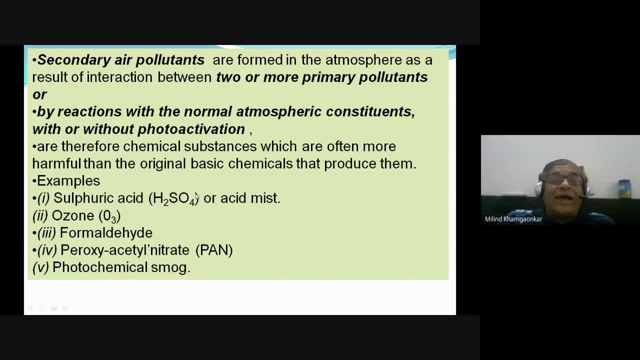 jada dangerous. hoega is, k example, a sulfuric acid, h2so4, or the acid mist, ozone, o3, formaldehyde, peroxyacetylene and acetyl nitrate, photochemical smog. okay, so all these are the secondary air pollutants. sulfuric acid, again, acid mist, it is mixed with. 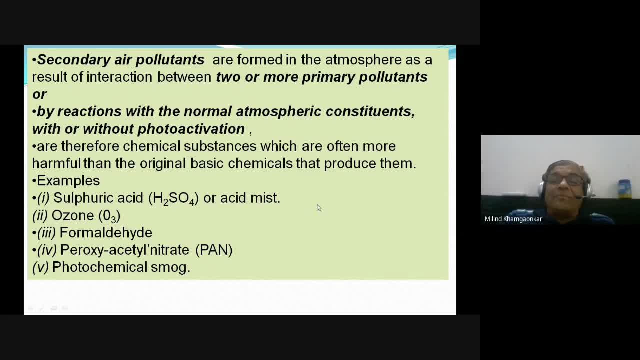 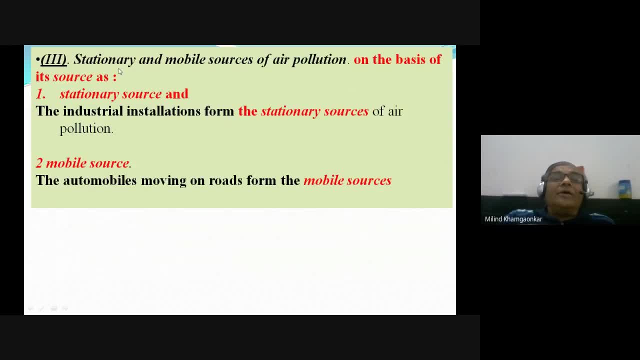 water or the vapor, then it is very harmful for the, as if it's a b 빠 bo heli remaining vapor. now studies are shown that surface, as a holographic septic lebels hawking the peripheral surface, has such strong effects. procedures follow it never. leave the surface as it has become more content, we are not seeing any kind of like things anymore. ohh, d'oh, ugh, please doesn't live and cut yourself, just look, just look now, this amazing culture of being a human being. actually, then, be humans, which are. 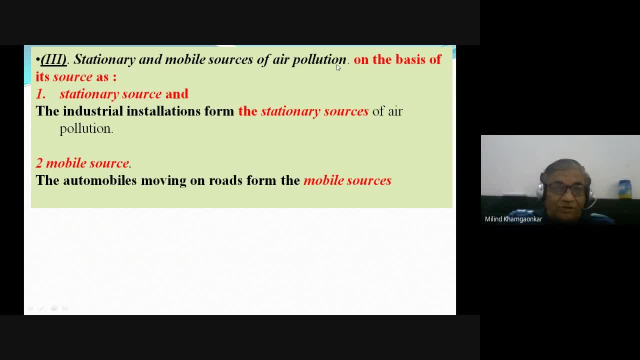 Stationary and mobile sources of air pollution. The stationary source means the source that is in one place, means from where pollution starts from one place, the source that does not move. that is called a stationary source, Like in our homes, individual houses. 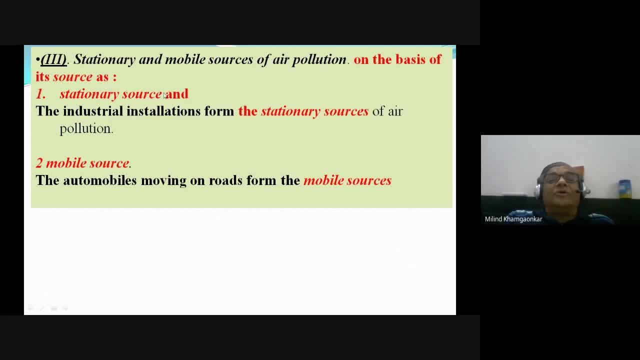 if we have a stove that burns wood, it is because of burning wood or coal, The gas that comes out of it, carbon dioxide and carbon monoxide, etc. or an industrial installation that cannot move from one place to another. it does not move from one place to another. 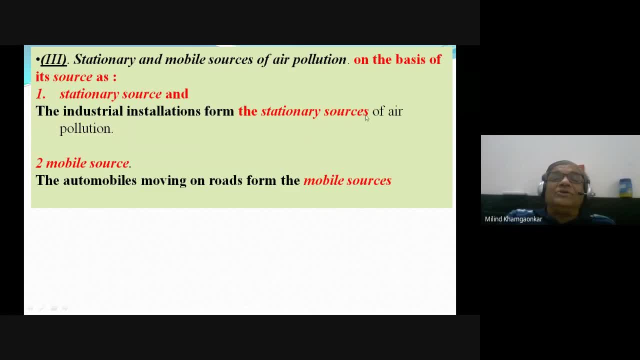 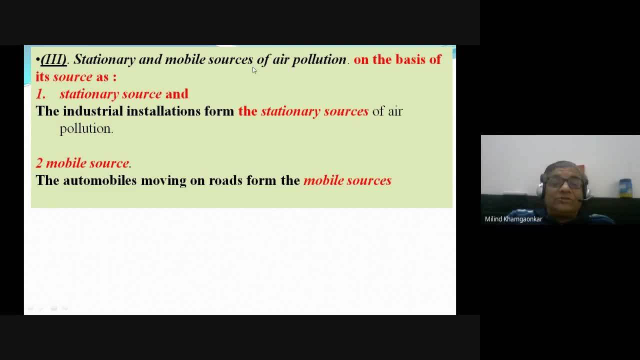 then you can very well understand the mobile sources. Mobile sources means the pollution sources which move from one place to another, That is, the automobiles. Our automobiles are motorcycles: cars, trucks, tankers, railways, aeroplanes, etc. Our automobiles are motorcycles, cars, trucks, tankers, railways. 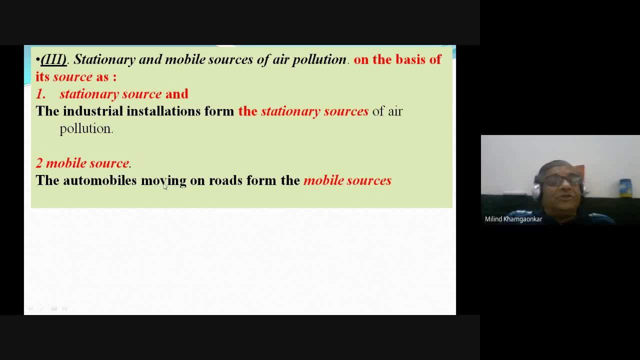 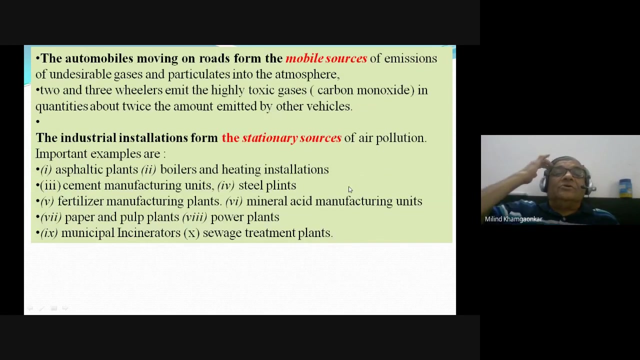 aeroplanes, etc. So these are all called as These pollute the atmosphere. They also produce the pollutants in the form of the gases, fogs, dust, aerosols. So the automobiles moving on roads form the mobile sources. 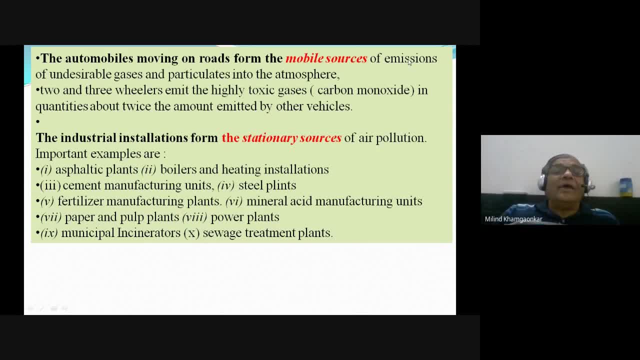 Because they have mobile sources. they have the emissions of undesirable gases And particulates or aerosols into the atmosphere. These mobile sources emit the non-required gases or hazardous gases And certain particles, aerosols into the atmosphere, which is actually harmful for the human being, for the animals. 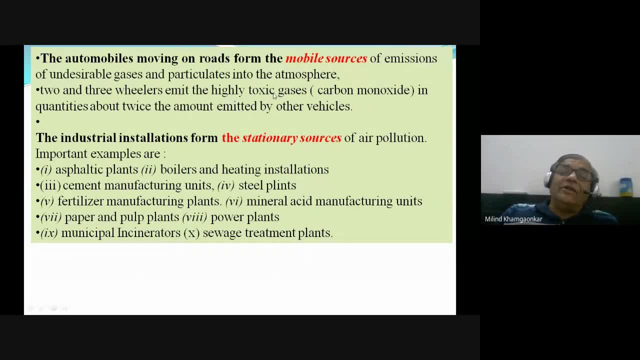 Two and three wheelers emit highly toxic gases. Four wheelers also. That is why there is a lot of control over this: Bharat 1,, Bharat 2,, Bharat 3,, Bharat 4, now Bharat 5.. 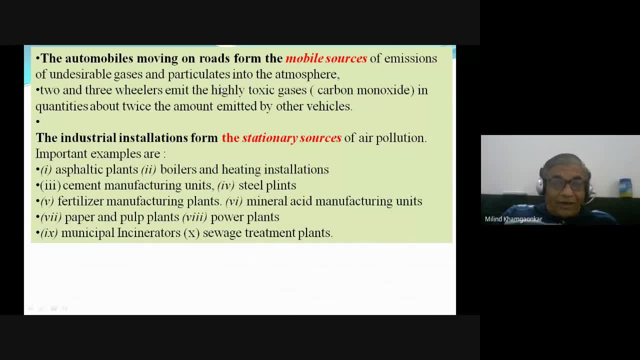 Emission norms. Okay, Again, what I am explaining. you try to understand in the present context. What is the position of pollution today. You will know that. If not, then you will know from the net What did I say, Bharat 1.. 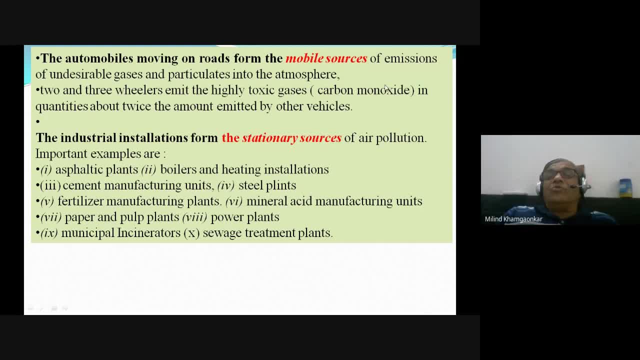 Or Euro. Euro is the standard Our motorcycles, four-stroke cars, etc. So Euro standard means European country, American standard, American country And our Bharat has its own standard. We have called it Bharat, Bharat 1.. 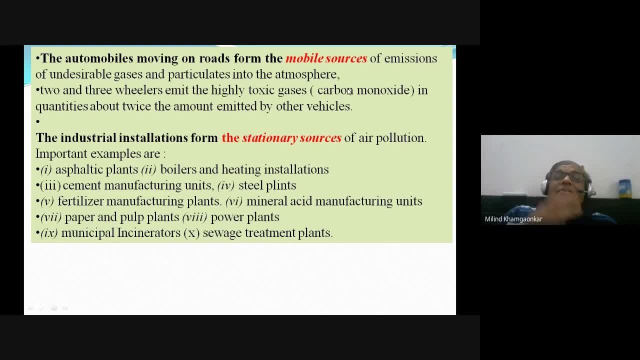 That is as you call it in the computer: First generation, second generation, third generation, fourth generation, etc. As the computer or the laptop goes on developing In the same way, the pollution norms are there By the- again- Maharashtra Pollution Control Board. 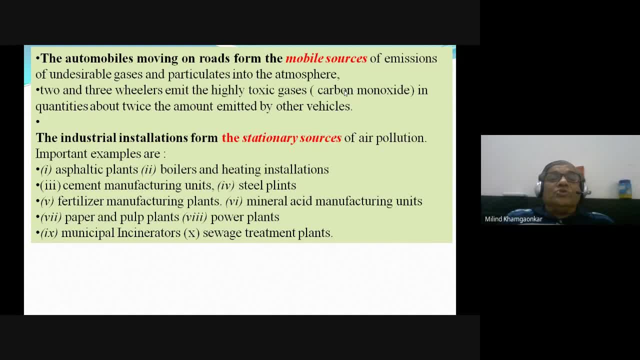 national level control board. So they have decided the limits of all those polluting gases- carbon dioxide, carbon monoxide, methane, et cetera- from the two wheelers, three wheelers, four wheelers, etc. And nowadays more attention is given on all this air pollution. 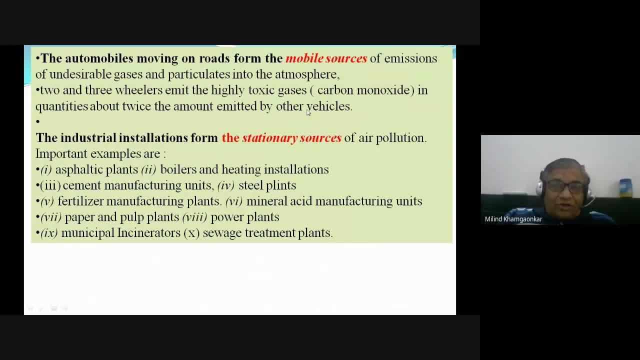 So what is the norm now? Now, Bharat 5.. The latest generation norms of India is Bharat Five Vehicle. That is why, if you are a regular reader of the newspaper or the news around you, you must be knowing all these thing. 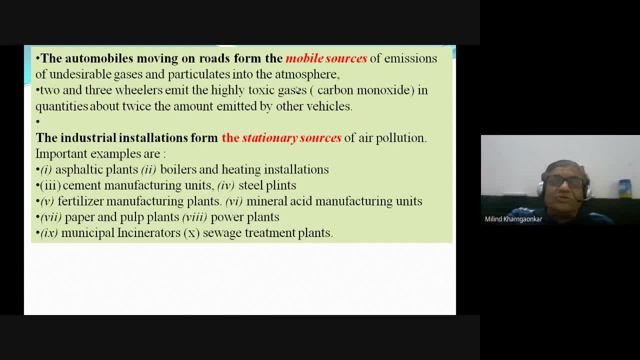 If you don't read the newspaper, don't see the news, do the beholding, you will not be able to identify. It will be clear to you that what's happening- whether it's happening or not, will be clear to you. 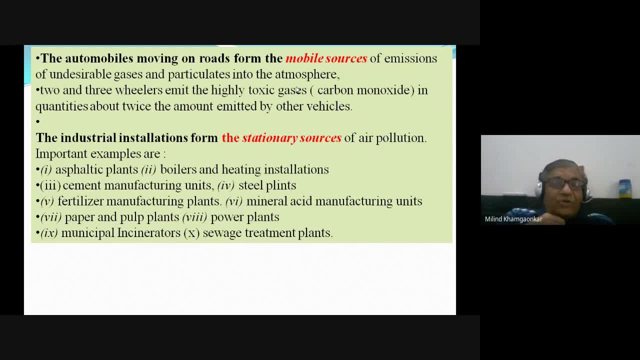 It is also clear-cut. It is clear-cut. It is clear-cut. Only depend on your WhatsApp university, then you will not get any knowledge or information. If you want to be a knowledgeable person, depend on the newspaper, depend on your Google, depend on your news on the TV or on the radio. 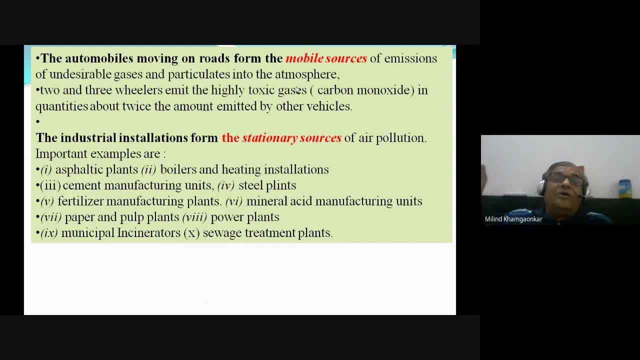 We can't keep good things in our mind. We watch news about Corona and Arona and make ourselves nervous, But, like I said today, the sky is the limit for the knowledge. And if you are an expert in one side, either just this subject, environmentally, or the treatment of the sewage. 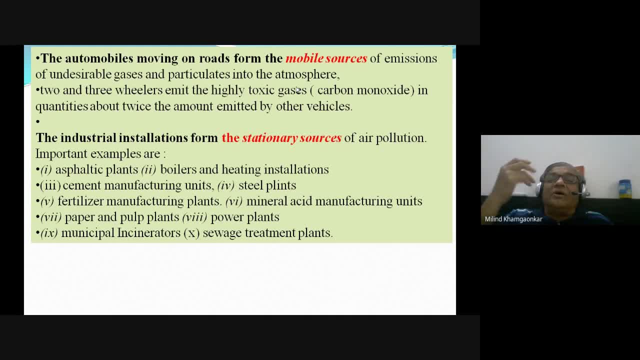 or air pollution treatment, or the solid waste treatment or whatever it is. so you can be a master and you can be a consultant there. So this is what I mean to say regarding the mobile software: Even though if a mobile solution comes forward, then I can use the existing encryption techniques to help younger people. 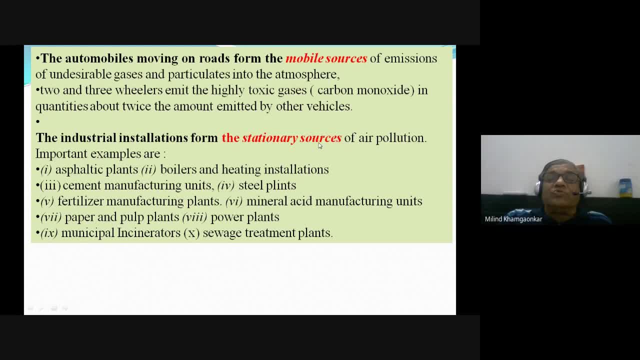 if I can use the technology that is available on the free network, then I can 아니라 mean there will be no by-evaluation work, But even so, this batch of devices can Kurban Infrastructure It has to do. Where will I put this camera? 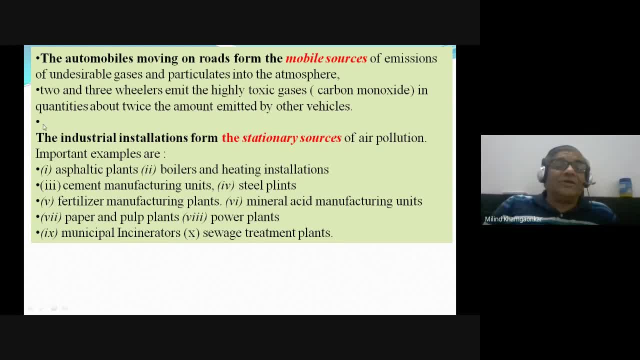 So the turbos are familiar with it. There's no mobile link to it. PI Highness metal mix for road work, boilers and heating installations. many boilers are there where heating is done: heating installations, cement manufacturing units, if you recollect what I have told you. 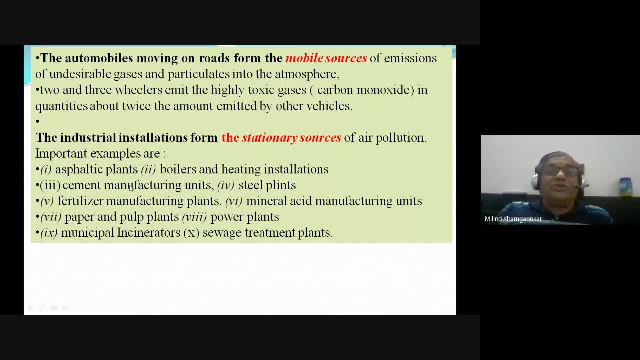 at that time 100 tons of the cement. if 100 tons of the or 1 ton of the cement is produced, then 1 ton of the carbon dioxide is produced. it is approximately 800 kg. so we can round it to 1 ton that 1 ton cement produces. 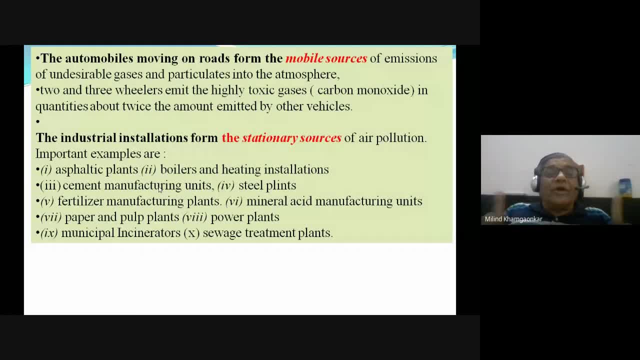 1 ton of carbon dioxide. that is pollution. so how can? the cement industry is dangerous for the air pollution, you can think. or the concrete industry? this is the pollution in cement manufacture. what is the pollution in preparation of concrete? what is the pollution in laying and compacting concrete? 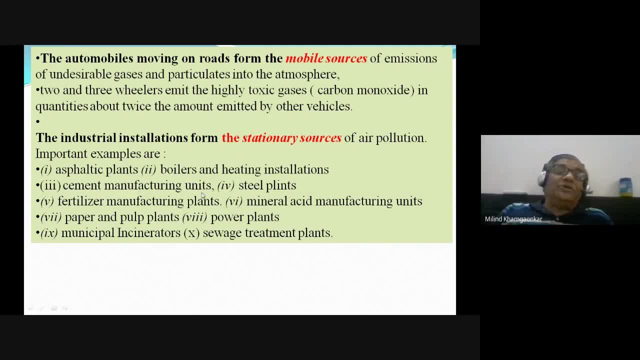 that also you can learn. so cement manufacturing unit is the example of the stationary source: steel plants, fertilizer manufacturing plants, artificial mineral acid manufacturing units, paper and pulp plants, solar plants, thermal power plants or any other type, but the hydro power plant does not create any hazard. that is the most greenest. 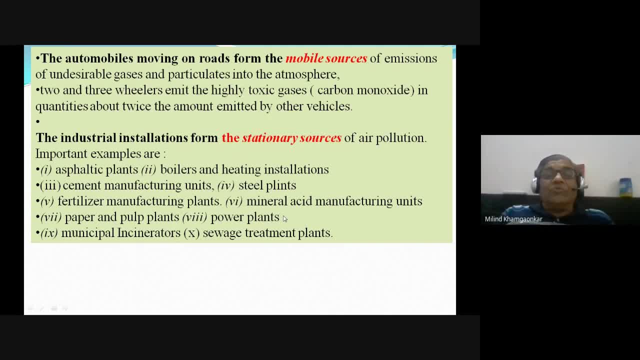 form of the energy that has been produced, so the more emphasis should be non-conventional energy: water. can you name other two types of the energies that can be produced? one is the solar energy and another is the wind energy. so all these three forms natural, that is the water. 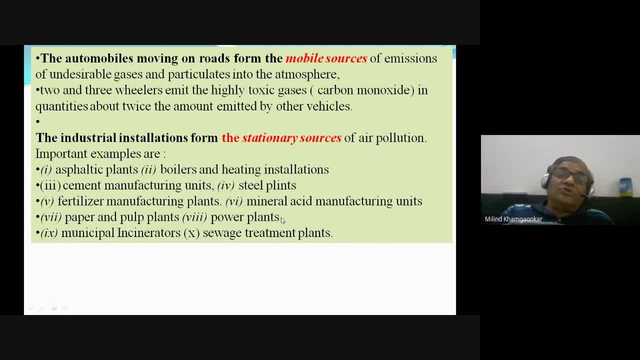 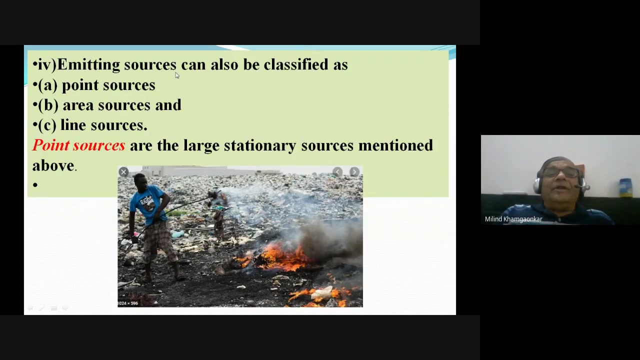 the solar and the wind, and also nowadays, the electricity is produced from the sea waves. so these are the alternatives to the power plants: municipal incinerators, municipal incinerators, wind water, ocean oil and so on. one who is in charge of the water and those over 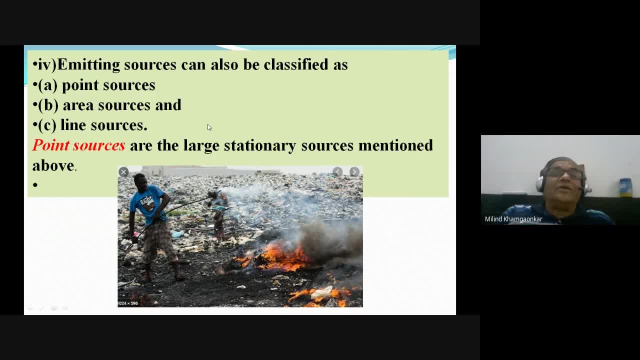 the surface of the area on the ground. here The pollution emitted from one place is called a point source. Emission from a very large area is called an aerial source. Like a train or a bus or a car goes through a road, that is the source of the line pollution source. 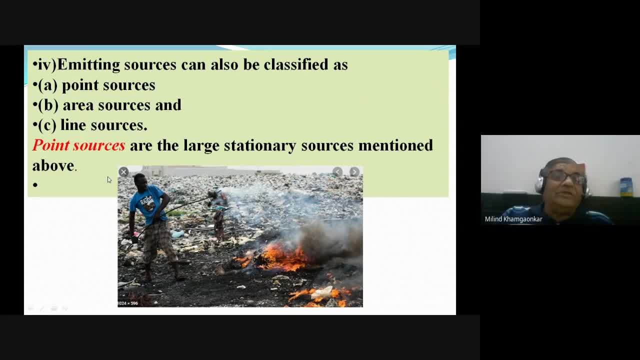 So point sources are the large stationary sources. The industries mentioned above are called point sources. Emission from one or the other house is called a point source. As you can see below, the place where we collect waste, there is a fire. 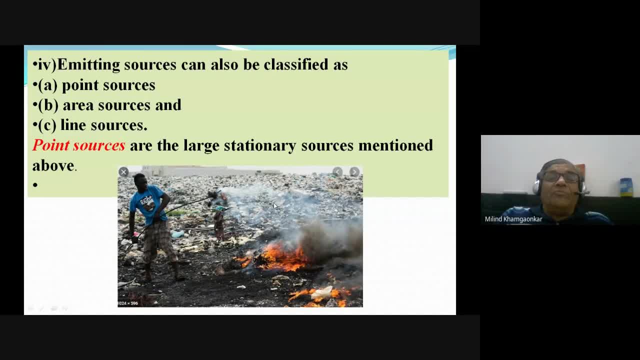 You must have seen this in many places In your village, in Nagpur, in Bhandewadi, or wherever you store this waste, there is a fire, there is pollution, nobody cares for that and ultimately results into the danger to the human life which are living nearby. 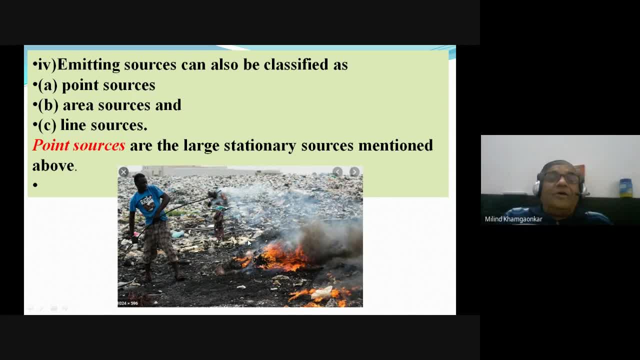 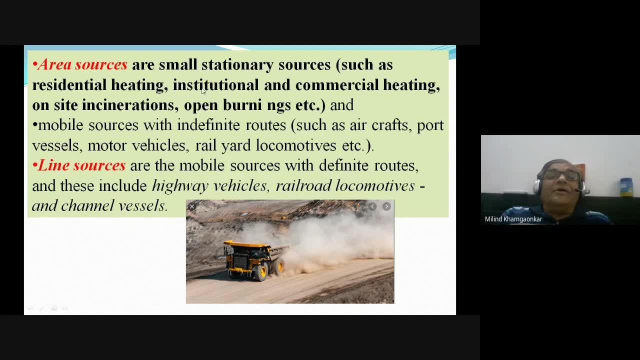 So that is the point. source, you can say Area source, like residential buildings, institutional and commercial heating, residential heating, on-site incineration, open burnings and mobile sources with indefinite routes, such as the aircraft, port vessels, motor vessels, rail and locomotives etc. 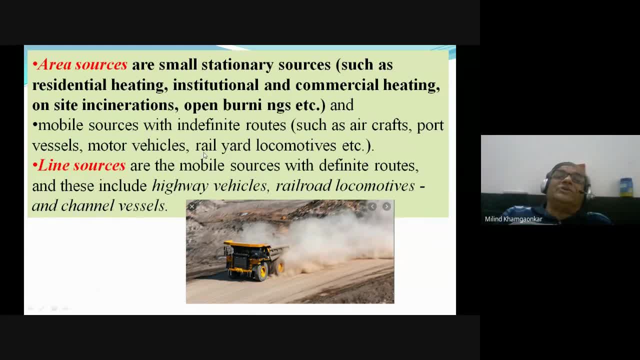 The pollution emitted from a very large area is called an area source, But of the stationary object, not of the moving object, Like in a village. in a village everyone burns wood to make a stove, So smoke will come out of the entire village. 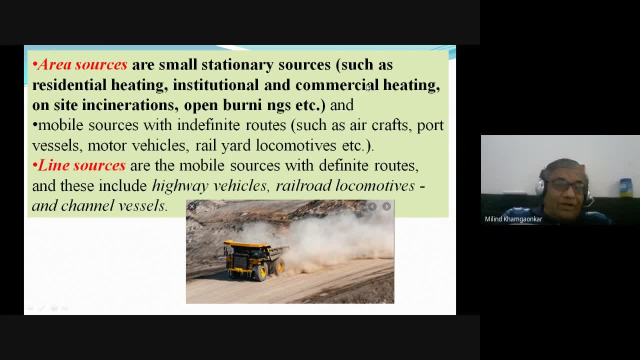 There is an institute, there is a commercial building. the pollution that comes from there too, because it is on the bigger scale. This is an area source. There is a residential area where there is a lot of burning. There have been a lot of such cases in Corona. 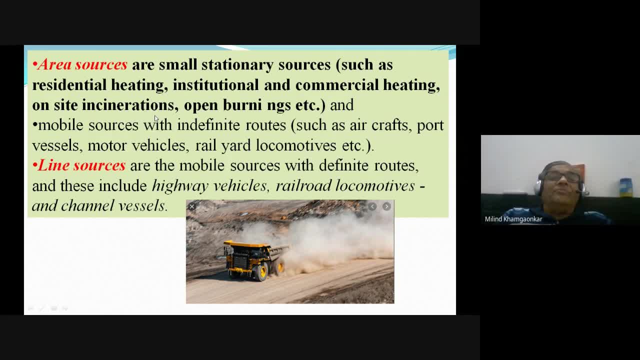 At one time. 10,, 20,, 30,, 40 people were burnt at a time, So that is again a sort of the pollution from the area. There are a lot of such cities, industrial towns, where a lot of concentrated industries are there, into that area. 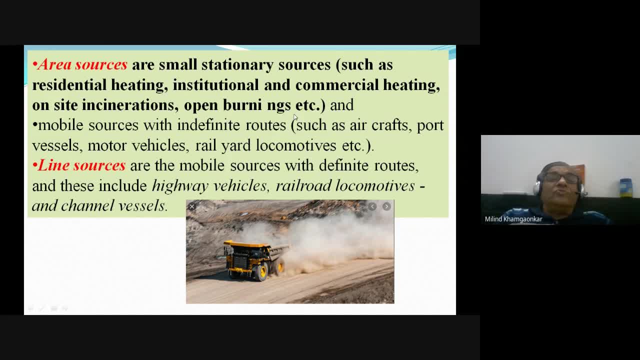 If you ever go from Tata Nagar by train, you will see that a lot of the steel industry is there, Very big industry, Bilai Steel Plant. So that is the area source, Line source, as I have told, the mobile sources with definite routes. 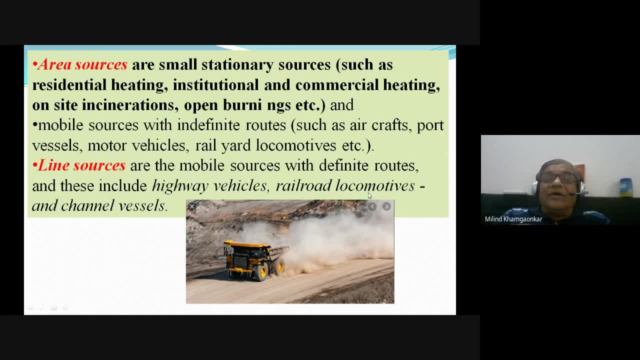 just like the highway vehicles, railroad, railroad locomotives, channel vessels, the traffic on the highway, as you can see in the road below pollution, Railway, the railroad locomotives, the locomotives that go through the railway. 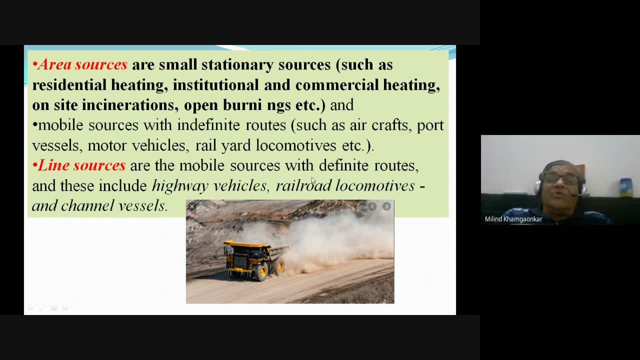 if it is electrical then there is no problem, But diesel, and today there is no coal, so due to diesel there is pollution. Electrical locomotives produce very less pollution, And from the river, from the sea, from the lake, 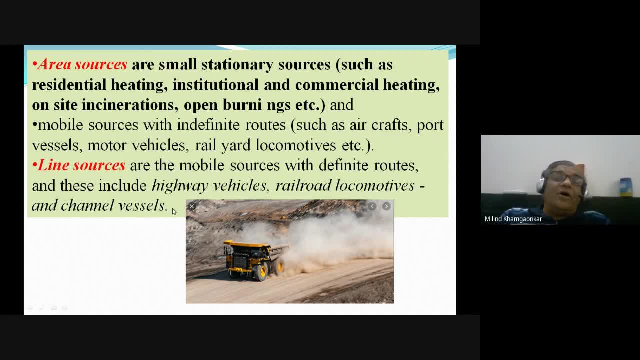 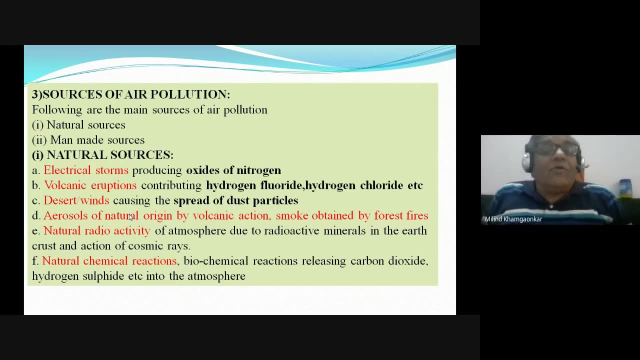 vehicles, when some boats go again on the combustion of the coal or combustion of the diesel, etc. that creates a lot of the pollution, So that you can say: is the line pollution? Now, various sources of the air pollution. 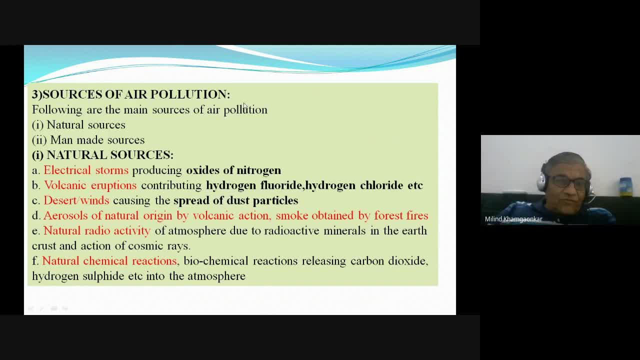 we are moving to the next part, That is, sources of air pollution. Following are the main sources of air pollution: The natural source and the man-made source. As I will again remind you, friends, very regularly the short notes are asked on this topic. 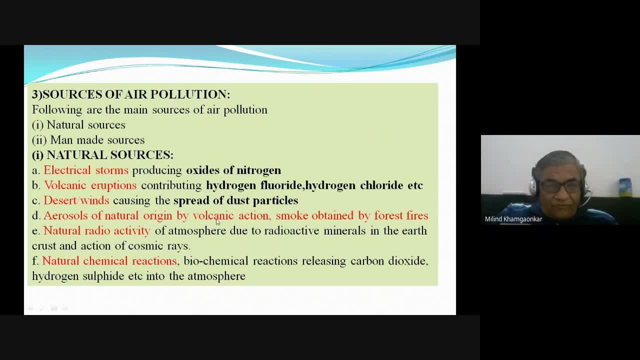 on this discussion we are having, And if MCQ will also be there, then that will also be based on all this, what we are learning or moving ahead. So not only listen, but try to note it down, try to jot it down. 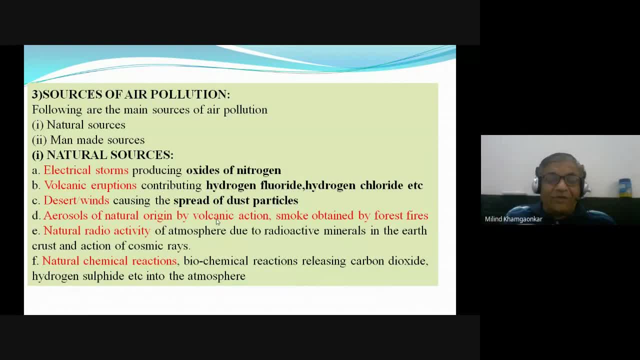 And also it will be again my request to all of you to please go through the earlier video recordings. Again and again, I am telling you: go through the earlier video recordings, go through the lectures, go through the notes you have been given. 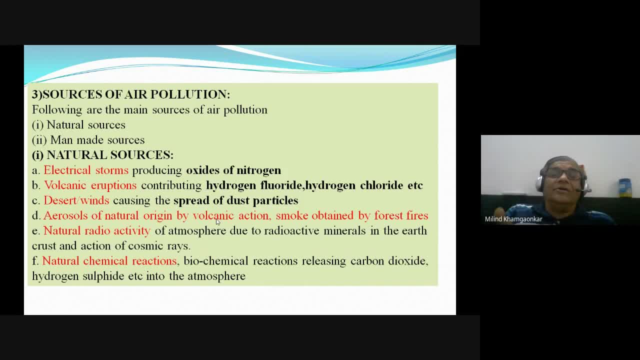 Actually, you are lucky that you are in such an institution like our college that you have been feeded by everything, Just like spoon feeding. you are being given everything. You are being given notes, online teaching video. now you will also get MCQ questions. 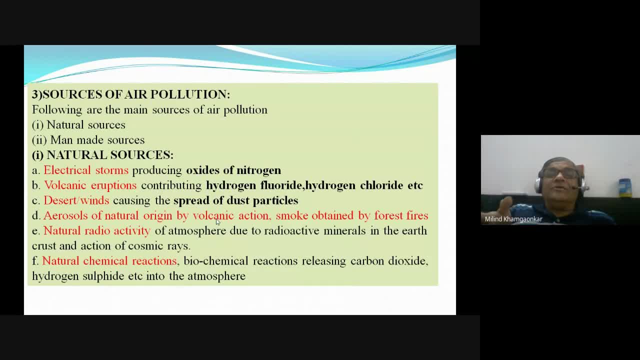 question answers, But still the attendance of the class is less, Attention of the student is less, Ambition to the student is less. Therefore, these are the reasons We don't have any ambition to go ahead After telling you so many ways. 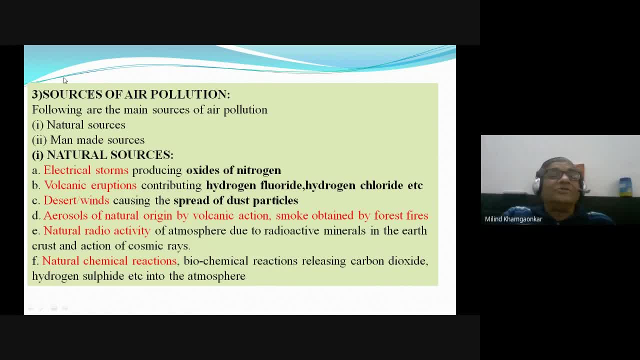 Okay, Let's move ahead With all these sources of the air pollution: natural sources, man-made sources. Natural sources are the natural. In the natural way there is pollution in the atmosphere. It is very important for us to understand that. 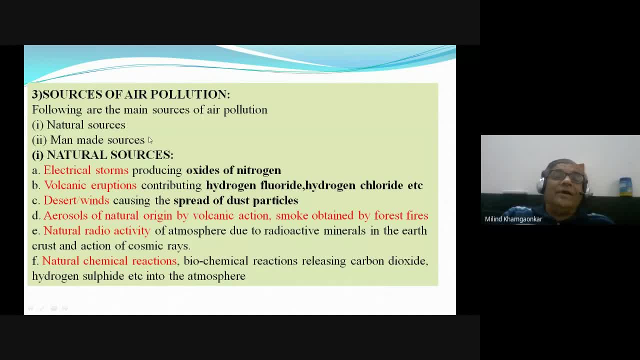 Many times. it is not so that man-made sources or human-made sources are very large, But there are natural sources. If man would not have been on the earth, there will be pollution, But that is natural pollution And the nature has got the tendency. 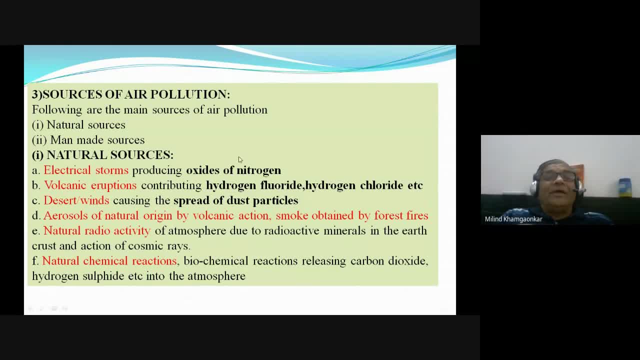 to again adjust it. It can be adjusted, But the man-made pollution is very difficult to adjust by the nature And then it affects the human being. Then we are in trouble. Okay, Corona is the very good example. It is the biological pollution. 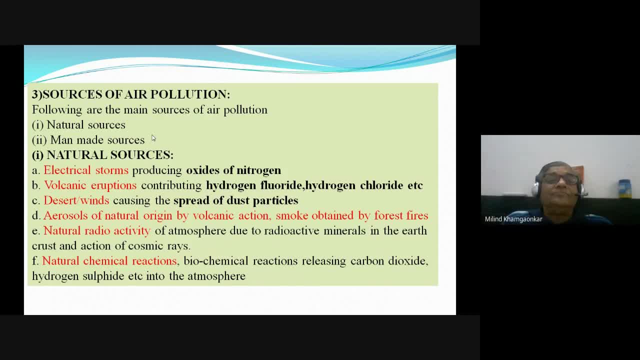 created by one of the country And all we are suffering for that. All the world is suffering. You are suffering, myself suffering. all around us, everything is facing the problem, from their life to their livelihood. Corona has affected their life and their daily earnings. 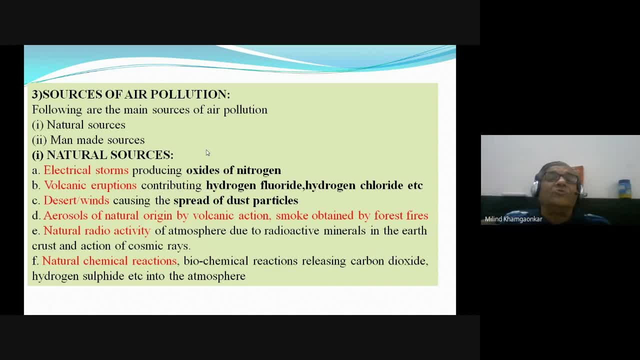 But again, I say that, without being nervous, you make yourself competent by using all this time, Because this is going to end after six months. But that is man-made source. So natural sources are the electrical storms producing oxides and nitrogen. 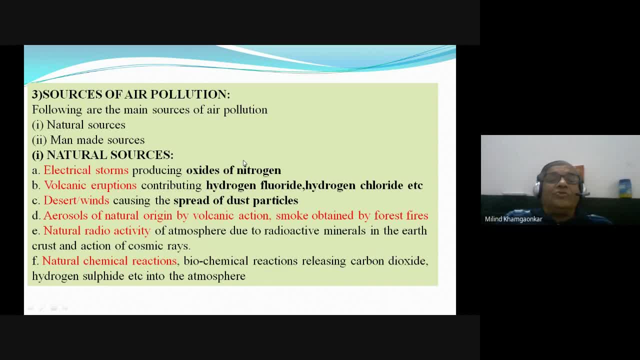 Right. When it rains, we call it thunderstorms, Thunderstorms, And they are also called as the electrical storms. When it rains, when electricity falls on the earth, that is one of the source of the electrical: by the natural, by the nature. 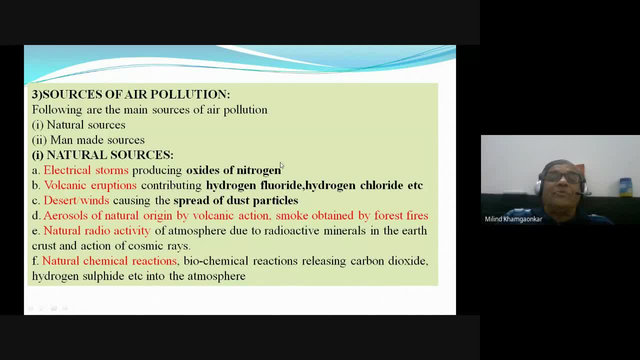 in which the oxides of the nitrogen are produced. Okay, And they disperse into atmosphere NO2,, NO3, etc. And if this NO3 mixes with the water, then the nitric acid will be produced. So we call it as the acid rains. 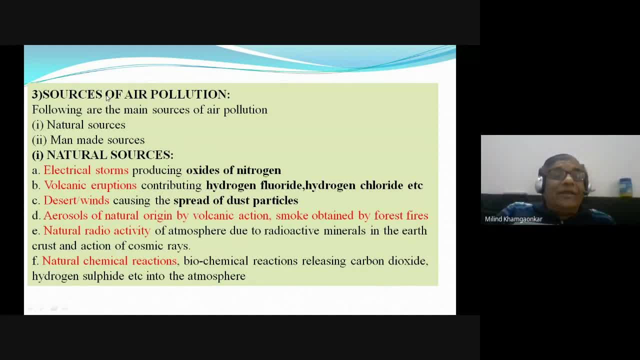 Occurs sometimes. So that is the electrical storms, That is the electricity Or the thunderstorms. we call it Volcanic eruption. I told you that when the volcano erupts, when the volcano erupts, when it comes out. 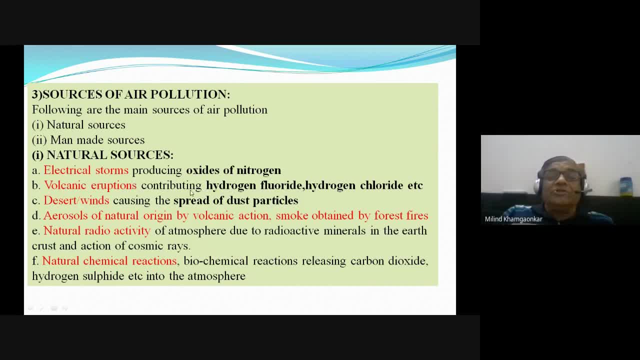 then from that contributes a lot of the hydrogen fluoride, HFL, hydrogen chloride, HCL, and a lot of the dust also. So so that is the natural resources: Desert winds. our deserts are called in Palavant Marathi. 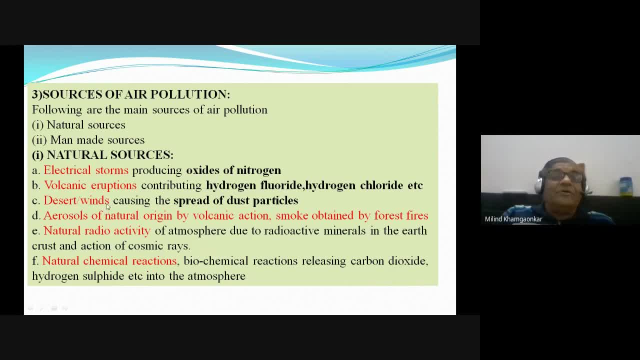 in Hindi I don't know exactly, but in Palavant Marathi it is called desert winds, So in Hindi- I don't know the exact word- deserts like in Thar desert or in Rajasthan and so on. 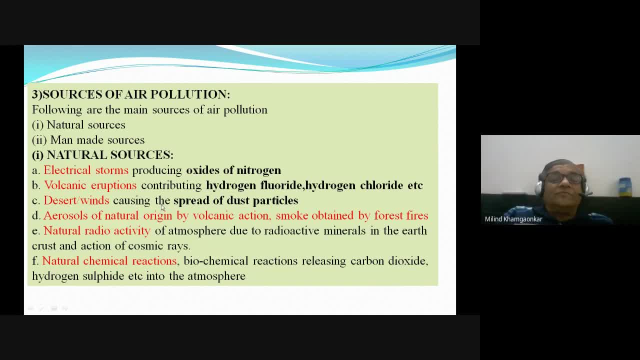 So from those deserts a lot of air flows with force And that air is spread, along with the dust, Our Delhi, our national capital, if in Dhupkale or around that area, Delhi, because it is very near to. 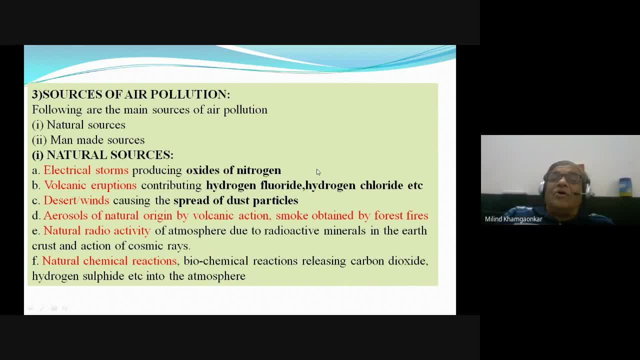 or it is on the southern part or on the western part of the, on the eastern part of Rajasthan, that Delhi receives a lot of the dust clouds. in the summer In Delhi there is a lot of dust pollution, And in winter 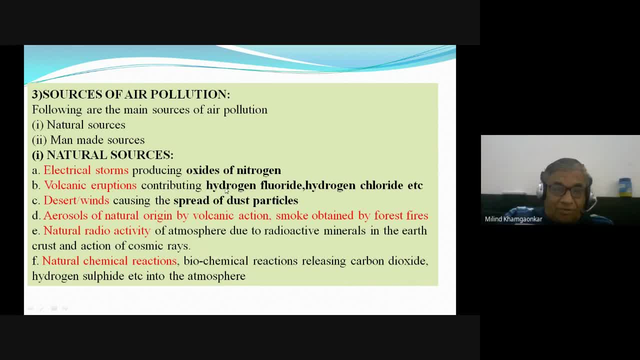 people after winter burn the garbage in the fields Before winter and after winter. there is a lot of pollution in Delhi. That is why you must have read in the paper: Delhi faces a lot of the pollution. So the desert wind. 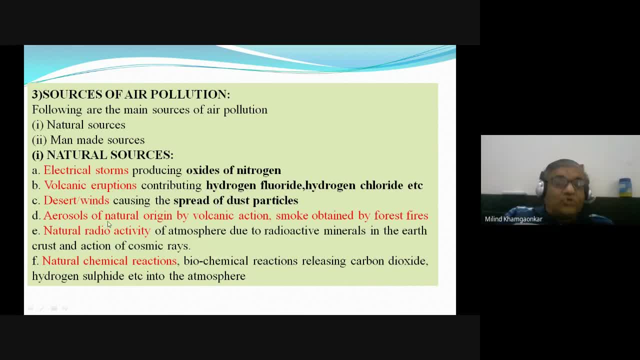 is one of the cause. Aerosols of natural origin by volcanic action. smoke obtained by the forest fires is also one of the causes for production of the aerosols. What does aerosol mean? The organic matter which is in the air, which is not visible through the eyes. 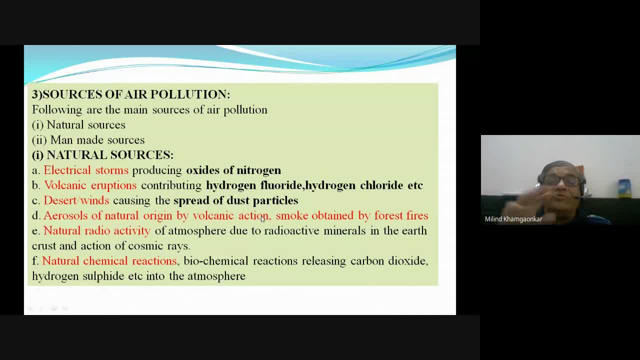 But if we inhale them, if we inhale them through our breath, then our lungs, or if we have an allergy, then again it may create the asthma or the asthma and also the TB, also of the tuberculosis of the lungs. So aerosols, 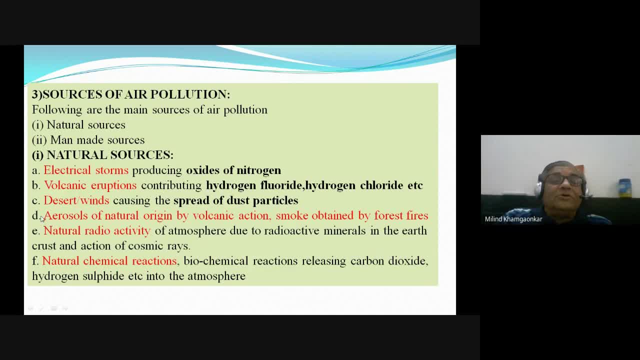 of natural origin by volcanic action, from the fire or the smoke obtained by the forest fire, the jungle from which the air comes out, that is the natural source. So aerosols of natural origin by volcanic action is also a problem. 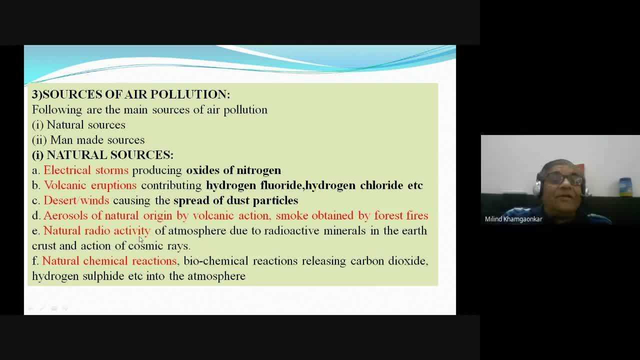 But aerosols source, natural radioactivity of atmosphere due to radioactive minerals in the earth crust and action of the cosmic rays. and a sewerage says I'm a boat, sorry. electromagnetic views. the rails cover the race comes in the form of the electromagnetic waves and those are the some infrared rays, etc. 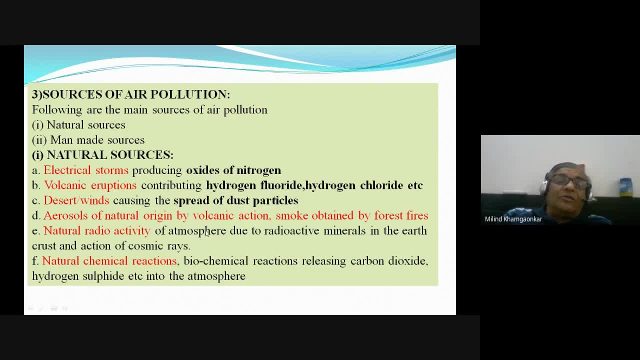 yd-os onkan layer around the earth reduces, then that may cause the penetration of those ultraviolet rays, he certain radioactive rays etc. on the earth and will burn our skin and may result into the cancer of the skin, also naturally occurring radioactive material on the earth also produces. 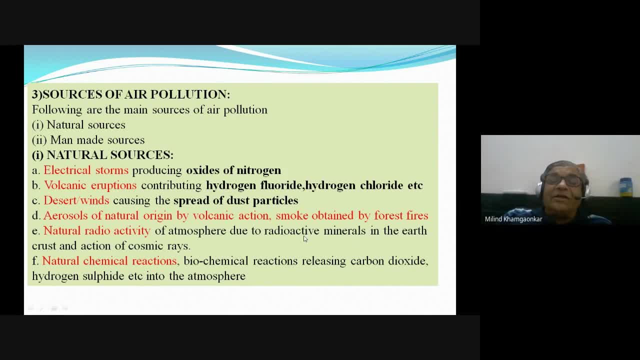 zrobić la luz y раз. però tant que las rayas radioactivas no crean la luz pero no se producen, una случida ad天 ni whoa información natural que ocurre en la mainlanda: radioactive rays, alpha rays, beta rays, gamma rays, etc. they are harmful for the 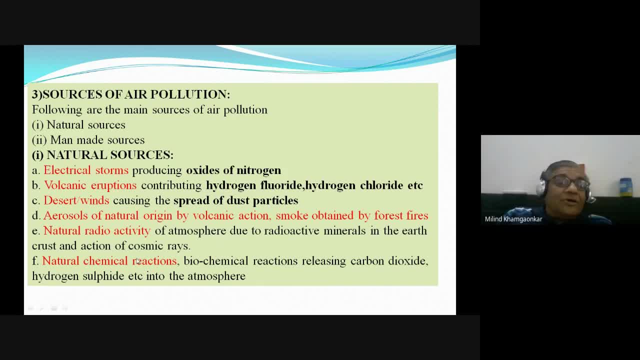 human being. so that is the natural radioactivity, natural chemical reactions, the biochemical reactions releasing carbon dioxide, hydrogen, sulfide, etc. into atmosphere. can you, can anybody? just a question. you can think and answer on your own, not are to me. what are the natural chemical reactions wherein biochemical decomposition takes place, releasing the carbon dioxide, hydrogen? 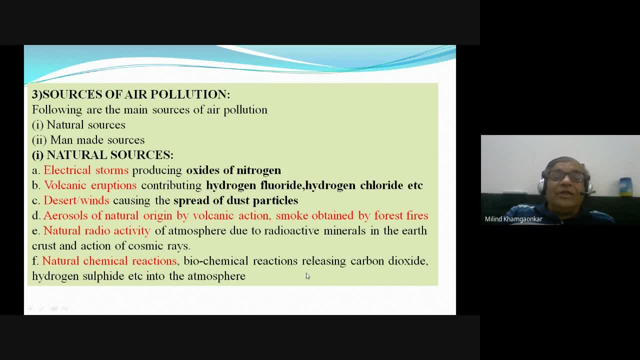 sulfide, ammonia's meet anything extra again, the decomposition of the organic matter by the anaerobic bacteria. septic condition, disco bolte churros, a hamper dr, a key by a Joe. organic matter, a organic matter, a organic matter, a containing certain from the vegetables, OHs from the human beings, human excreta. 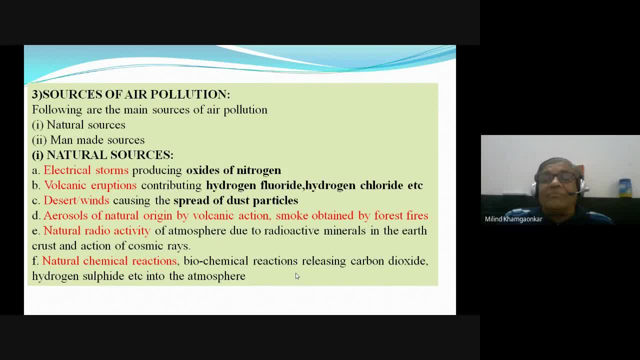 and all the material which contains the carbon. they are called as the organic matters. if they are decomposed by the anaerobic bacteria, puilty, sheable material is produced. two trees, she able, and a both, sir, a word of my both, specifically Barbara bhut. oh, and a both, sir, a word of my both, specifically barber both. 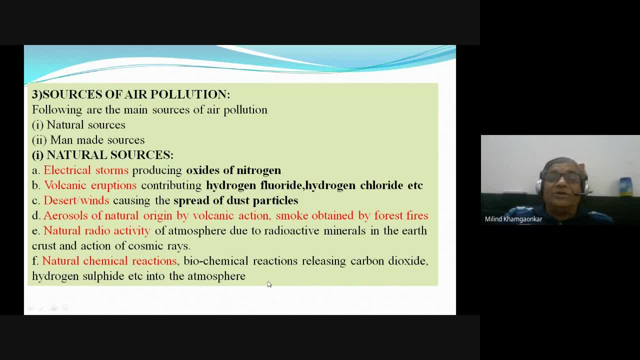 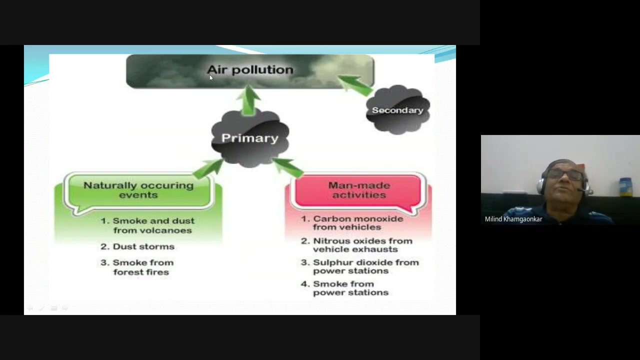 The foul smell is released through that, That is, in the form of the hydrogen sulfide. During that decomposition by the anaerobic bacteria, carbon dioxide is also produced, Methane is also produced. So this all occurs naturally. So therefore it is called as the natural chemical reaction. Again it comes under the natural sources. Again, schematically it has been shown: air pollution, primary and the secondary. 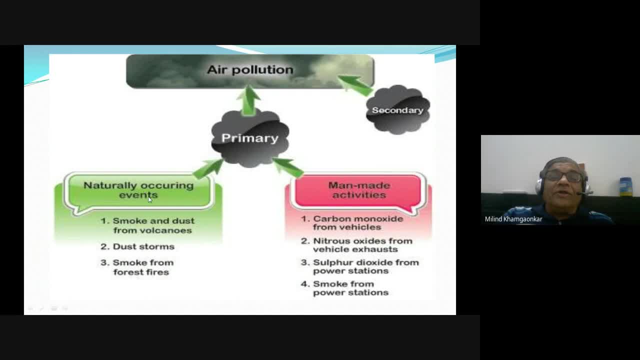 Primary air pollution- naturally occurring event and the man-made air pollution, Man-made activities, naturally occurring events, smoke and dust from volcanoes, dust, small storms like that occurs in the desert, smoke from the forest fires, And also here you can add the naturally occurring radioactive emissions or from the sun, that is, the ultrasonic rays, etc. 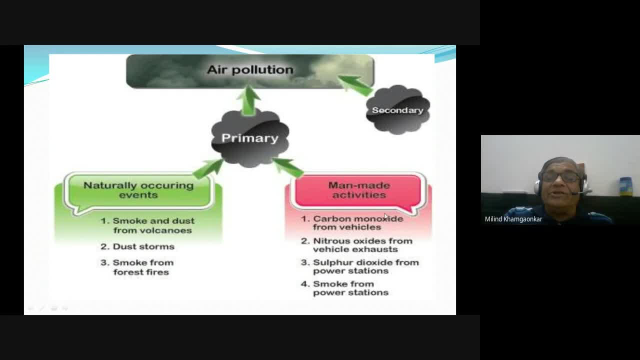 Natural occurring events, man-made activities, Carbon monoxide. from the vehicles- two-wheeler, three-wheeler, four-wheeler vehicles- carbon monoxide is produced. So therefore, the technology of vehicle is being advanced day by day.